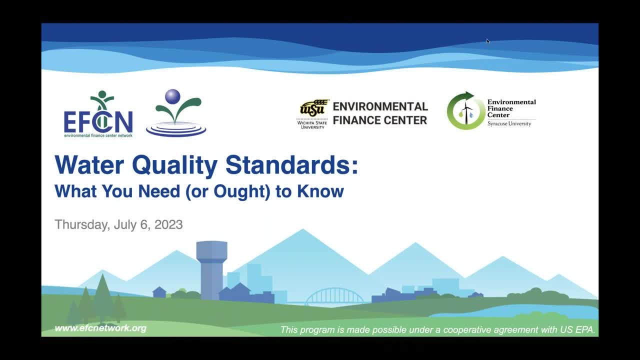 All right. Hello everyone and welcome On behalf of the Environmental Finance Center Network. welcome to our webinar on water quality standards. what you need or ought to know, My name is Kristin Crewe, from the Syracuse University Environmental Finance Center. Before. 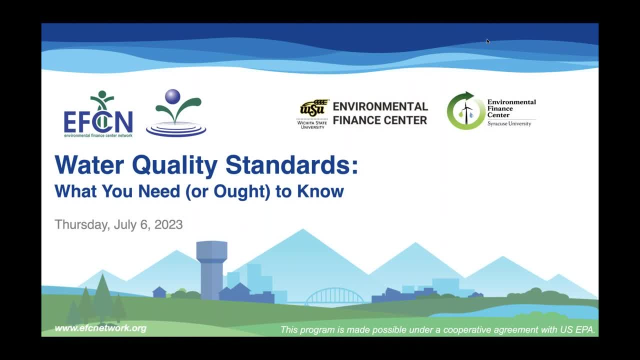 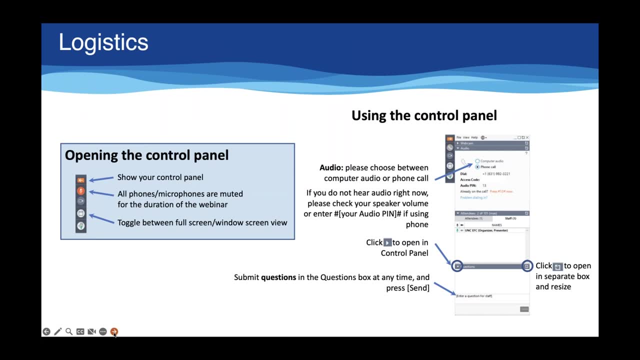 we begin, we're going to go over a few logistics and then we can get started. During the webinar today, everyone will be kept on mute to ensure audio quality. If you have a question, please type it into the GoToWebinar question dialogue box at any time throughout. 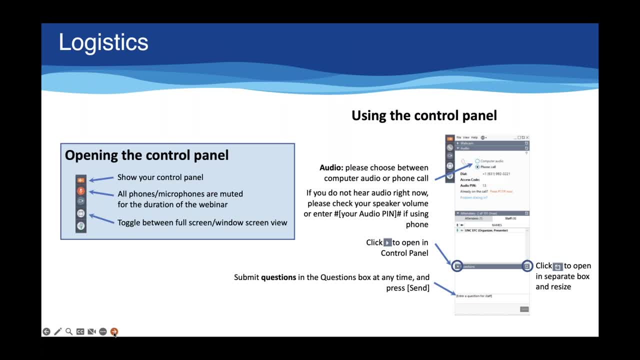 the session. We will be saving your questions for a facilitated Q&A session at the end of the presentation. After the webinar, you will receive a follow-up email that includes a link to the recording and other information that you may need. You're also able to download. the session from the link in the description. If you have questions, please type them into the Q&A box at any time throughout the session. We will be saving your questions for a facilitated Q&A session After the webinar today. everyone will be kept on mute to ensure audio quality. 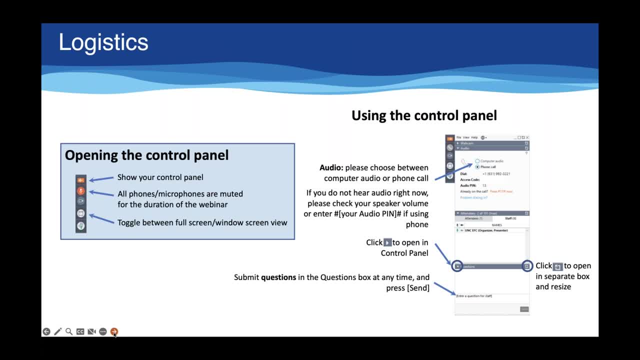 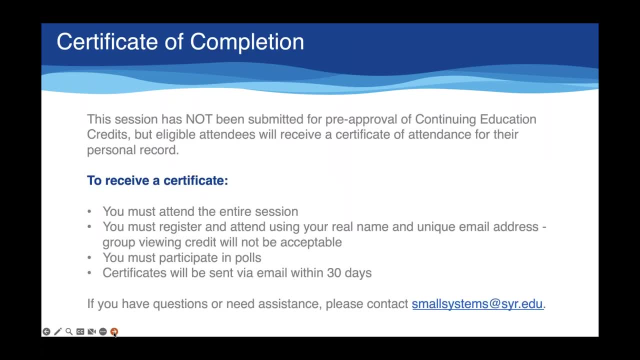 Before we begin, we're going to go over a few logistics and then we can get started. Before we begin, we're going to go over a few logistics and then we can get started. This webinar has not been submitted for pre-approval of continuing education credits, but eligible. 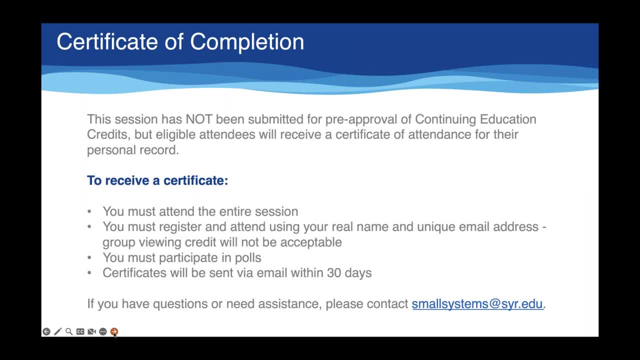 attendees will receive a certificate of attendance for their personal record. To receive a certificate for this session, you must attend for the entire session and register and attend individually using your real name and their Notepad name and unique email address. Certificates will be sent via email within 30 days of the 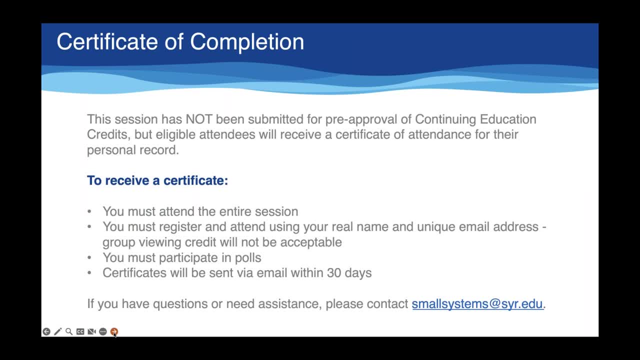 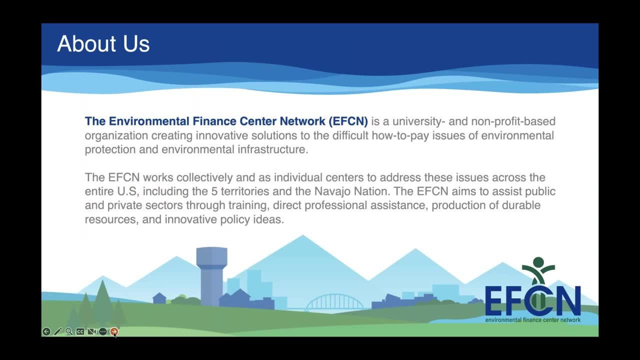 webinar date. If you have questions or need assistance, please contact smallsystems at syredu. Now for a little bit about us. The Environmental Finance Center Network provides training and technical assistance to small water and wastewater systems in all US states and territories through our Building Technical Managerial. 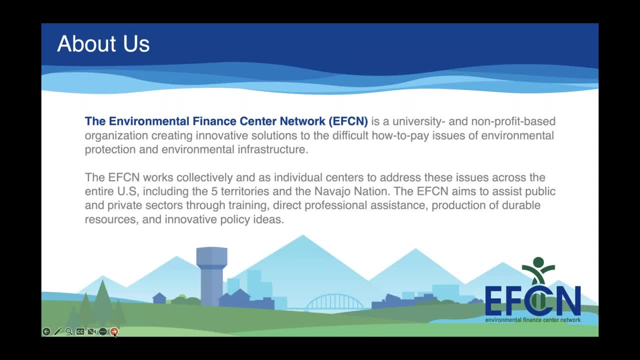 and Finance Capacity programs. If your community or utility needs assistance with drinking water or wastewater system management, please feel free to contact us through our request form, which I will be sharing in the chat very shortly. On that note, we can go ahead and get started. I would like to introduce our presenters. 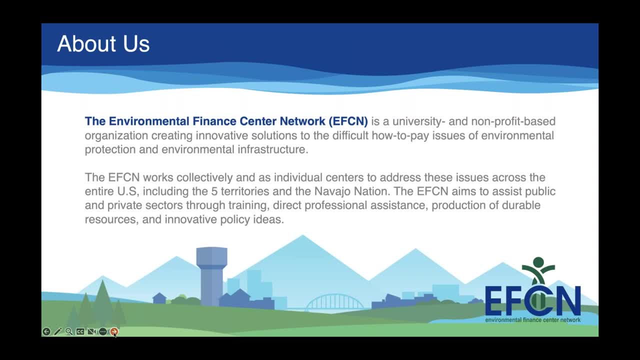 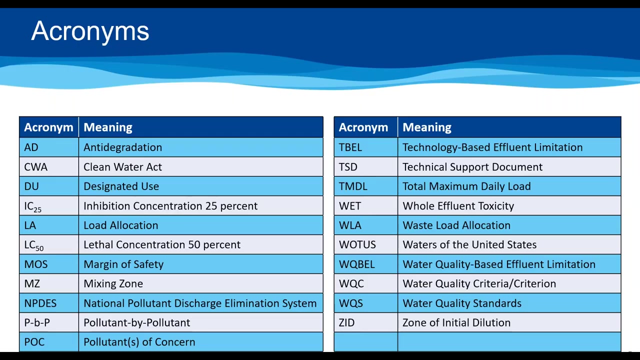 Mike Tate is an engineer and a project associate at the Wichita State Environmental Finance Center. Welcome, Mike, and I will hand it over to you. So, Kristen, do we have my screen? Yes, Mike, I can see your screen. Okay, Were you going to do the questionnaire or the questions? 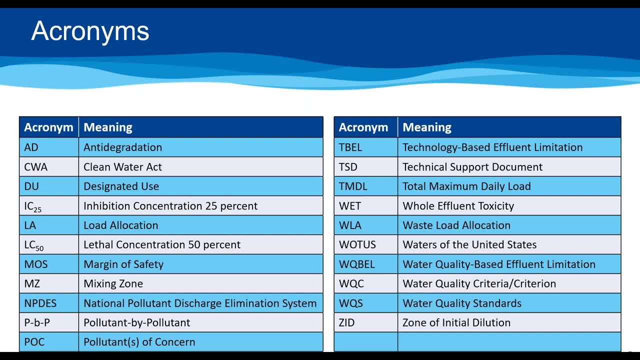 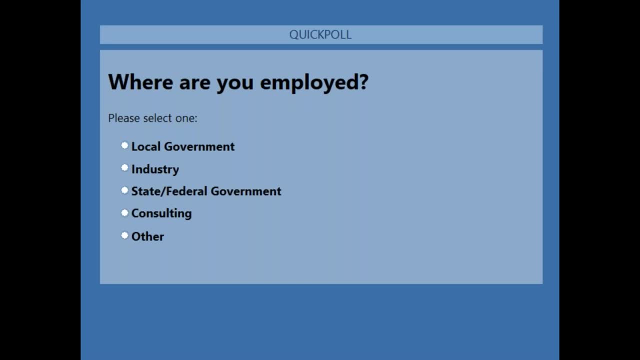 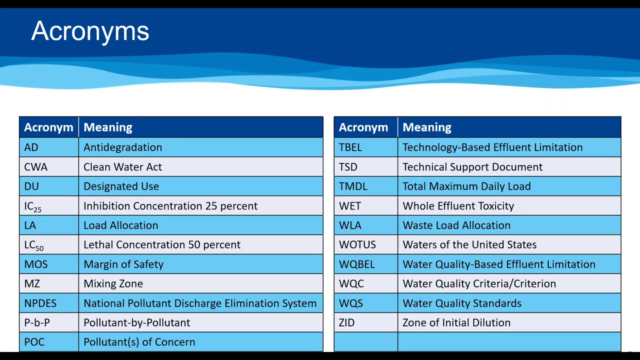 Yeah, We'll go ahead and do the poll questions. I'll send off the first one right now. Okay, All right, Everyone, where are you employed? Go ahead and get your answers in. I'll be closing the poll in three, two, one. All right, It looks like 45 percent are from. 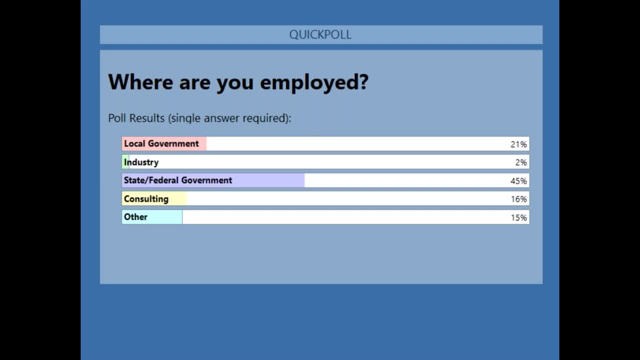 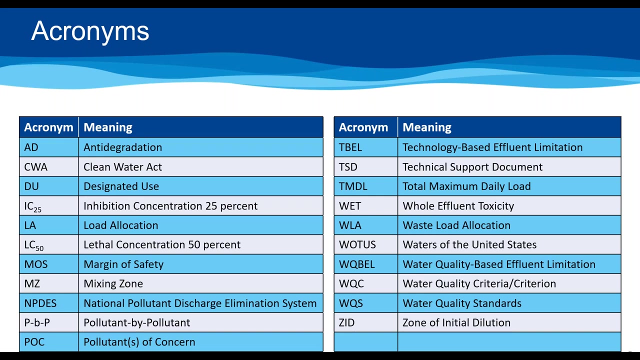 the state or federal government, 21 percent are from local government, 16 percent are from consulting, 15 percent are from other organizations And 2 percent are from the industry. So most people are here from the government. And the next poll: How would you rate your understanding of water? 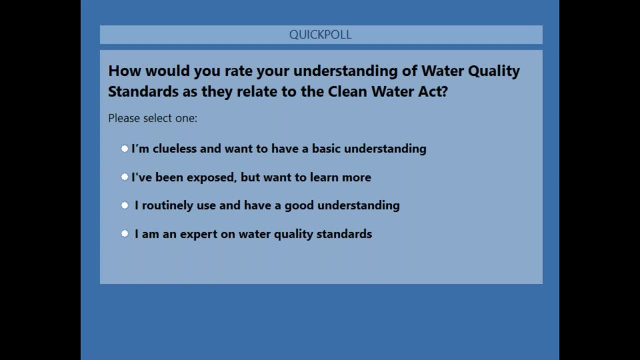 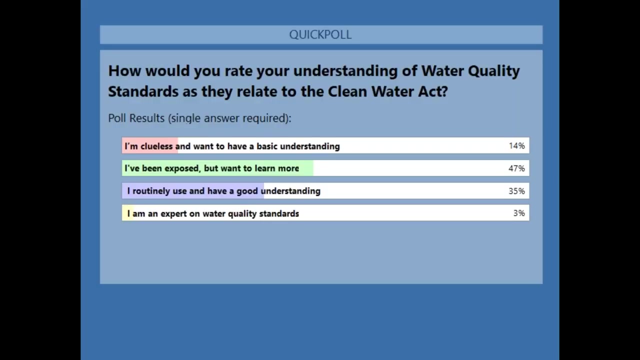 quality standards as they relate to the Clean Water Act. Go ahead and get your answers in. I'll be closing the poll in three. two, one. All right, it looks like most people have been exposed but would like to learn more. 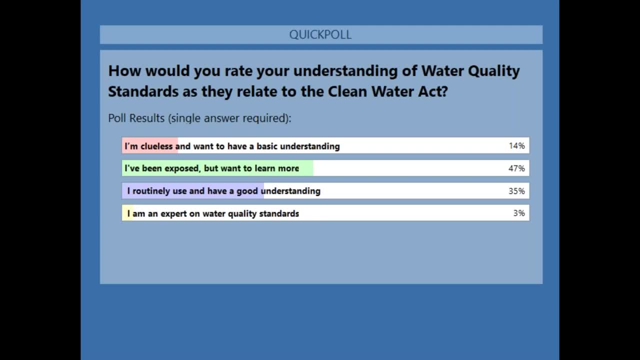 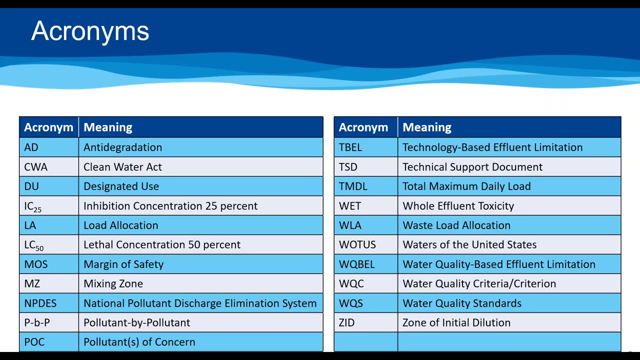 35% say they routinely use and have a good understanding of the water quality standards, 14% are clueless and would like to have a basic understanding, And then 3% consider themselves an expert. Okay, well, I won't be speaking to the 3%. 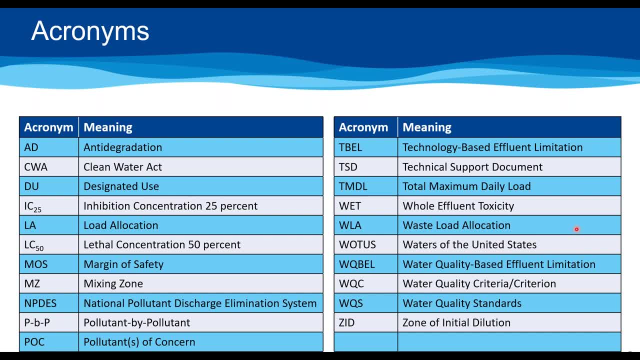 All right, is my screen displayed then? Kristen Looks great. Okay, all righty, thanks, Real quick again. my name is Mike Tate. As Kristen said, I'm an engineer. I work part-time with the Wichita State Environmental Finance Center. 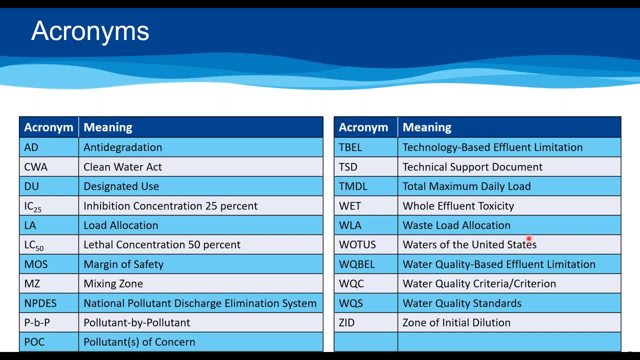 And just briefly about my background. I had 31 years of experience with the state of Kansas in the Kansas Department of Health and Environment, working mostly in the water area with permitting standards, drinking water, lots of different areas but all mainly involving water. 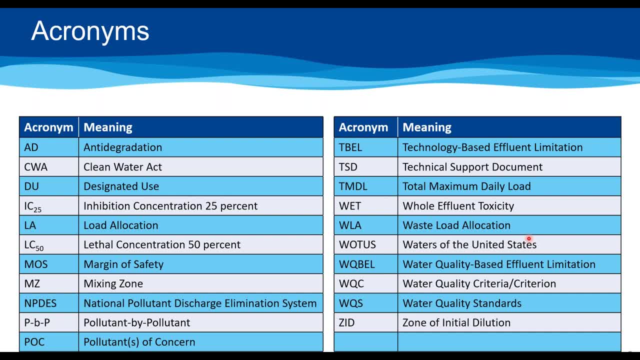 And after I retired from there I spent almost six years with EPA Region 7, before retiring from that. So I do have just a fair amount of experience with this stuff And hopefully I'll be able to share some of that with you. 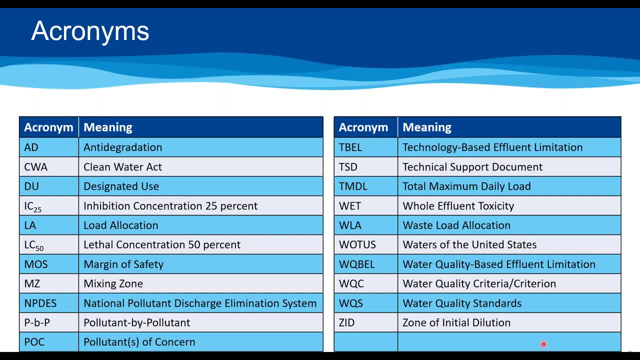 And hopefully I'm starting on the screen here that shows the acronyms that might be used today. This was a good suggestion that came from a previous webinar that it's an acronym-laden field that we're in, So we tend to use them a lot. 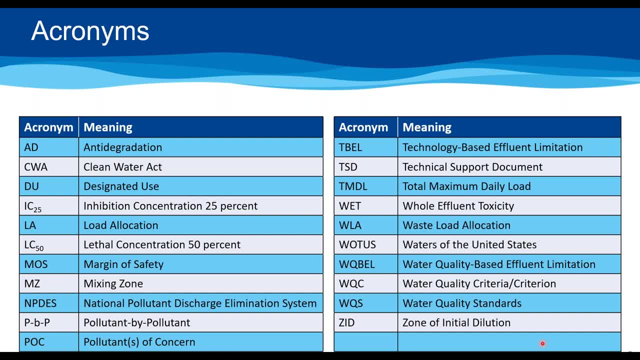 So try to put this up on the first screen And, as Kristen mentioned, you can download the handouts right off that tab on your screen. So if you need to have that, have it handy to reference back to the acronyms And then, if you're going to use it in the field, 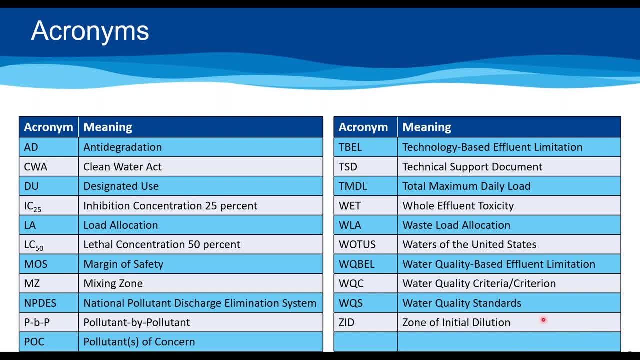 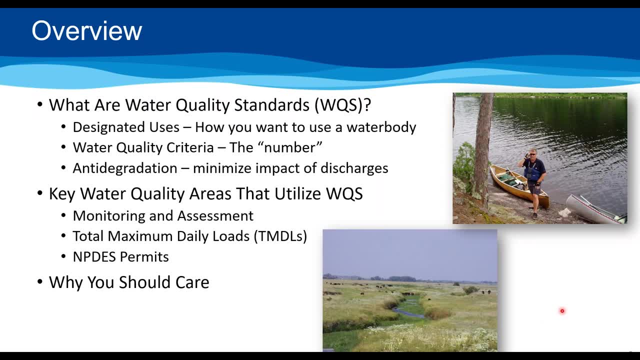 you can use the acronyms on the screen And I'll be able to link this up on the screen for you. Okay, So here's just a quick overview of what we're going to talk about today. It's you know. first off, what are water quality standards? 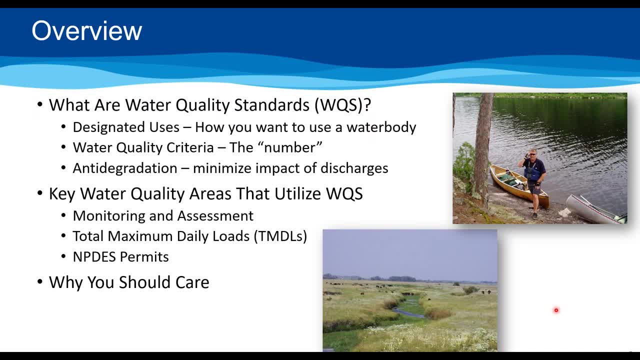 And just a little preview of it. It's designated uses, which means how you want to use the water body within that water body. a lot of people, i think, call that the standards. quite often it's really water quality criteria. and then the third part of the standards is anti-degradation. 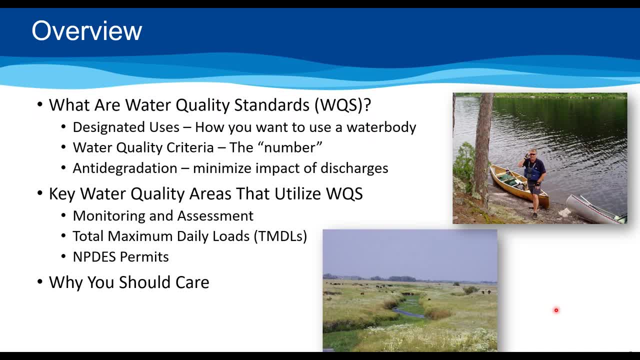 policy you use to minimize the impact of wastewater discharges on water. we're then going to talk about the key water quality areas that utilize water quality standards, and those tend to be the monitoring assessment programs that states have the tmdl programs. they run for impaired waters, and then for what? a lot of operators. 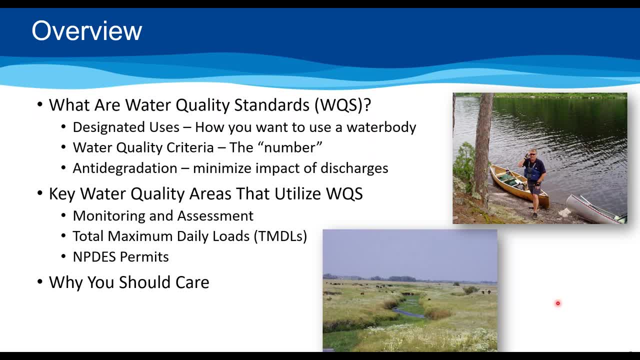 experience are in pds permits. and lastly, i'll try to give you some real world examples on why you should care about water quality standards. it can be a bit of a dry topic, it's. it's a lot to process, as i have at the end dpa sometimes. 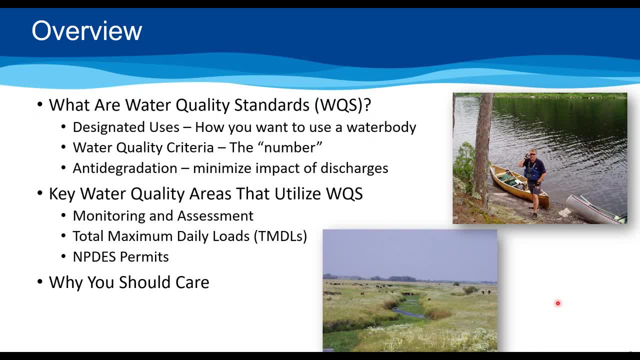 offers a five-day course on it. i used to work with the woman at dpa region 7 who worked with the standards and she said: boy, people aren't any good with this stuff until they've been here in three years, so you're going to try to learn here in about the next. 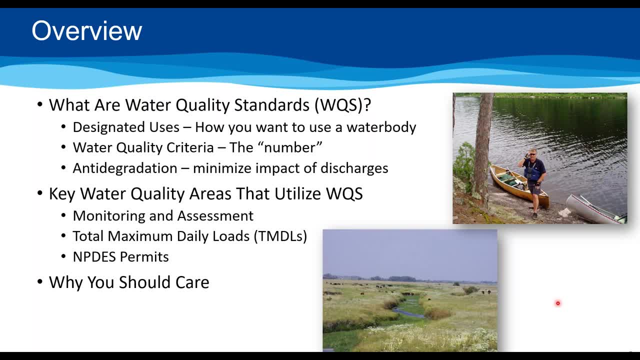 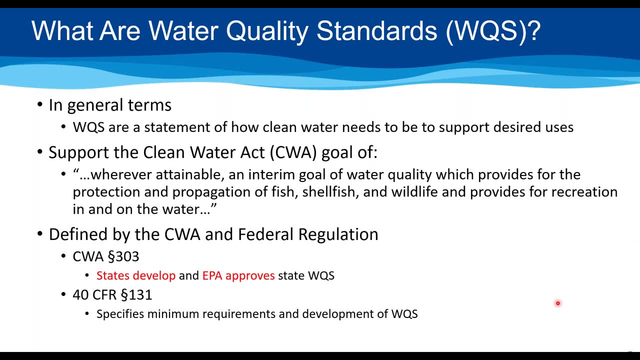 45-50 minutes. uh, what some people uh learn in three years. so i'll get going with it for right now. so that first question: what are the water quality standards? well, in general terms, the standards are a statement of how clean a water needs to be to support desired uses. 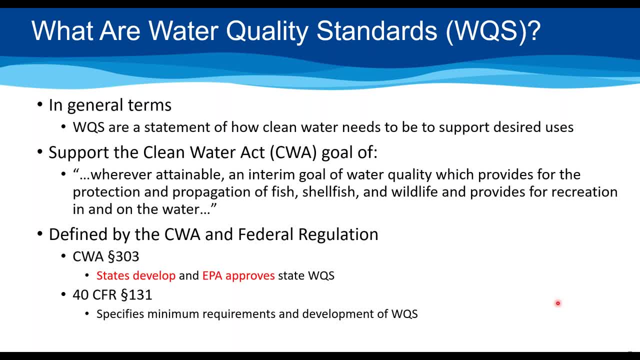 okay, so it comes right out of the clean water goals of the clean water act, right up front or you know, wherever attainable, an interim goal of water quality which provides for protection of propagation of fish wildlife. it provides for recreation in an online- okay, a lot of people you know you'll. 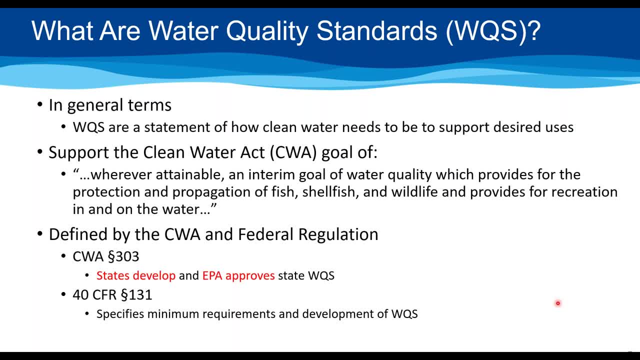 hear that referred to shorthand and it's fishable and swimmable water. those are really two uses of water. i will get into what some of the other uses are that states look at. probably a lot of them i've never even heard of before myself. but again, that's different from state to 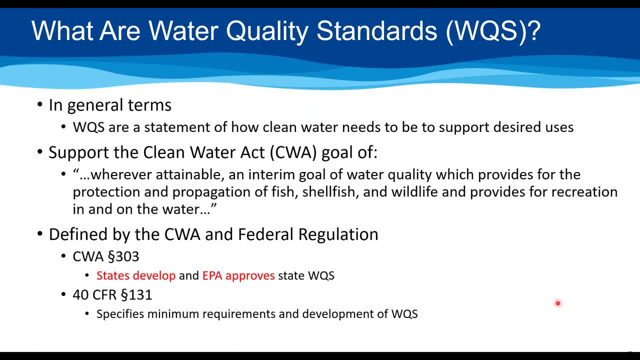 state and the reason that is is because of the clean water act. in this section 303 of the clean water act, it gave the authority to develop water quality standards to the states. it said the states will develop those standards, but it also gives epa the authority to. 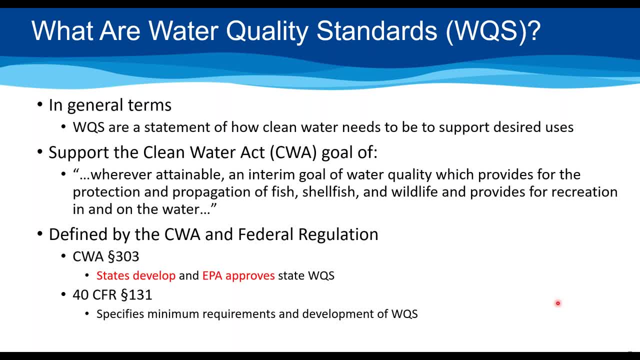 approve those standards for the state. so when you've got all the states territories, some of the tribes developing standards, you can pretty well rest assured that no two are going to be exactly the same. they're going to be a little bit different from state to state. a lot of the core parameters that you'll 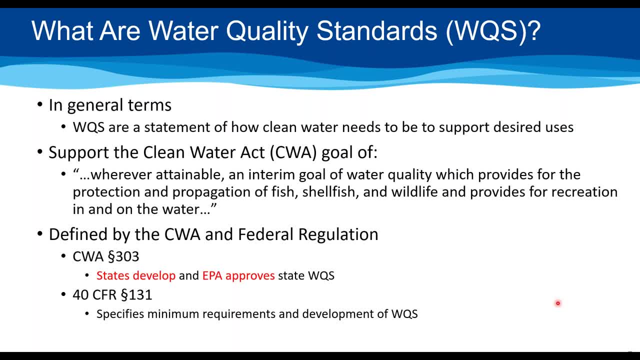 find in the standards are very similar from state to state. the thing they do all have to have in common is they have to have all of the elements of what comprises the standard. so uh, you'll then find uh later in the regulations. you can find everything you want to know about standards in section 131. 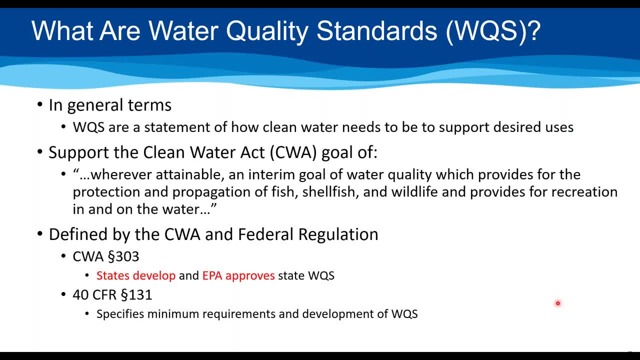 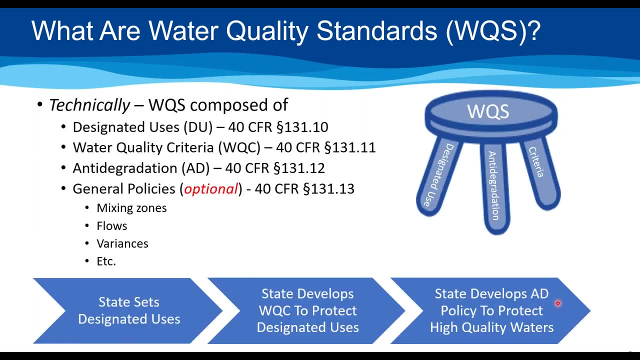 of part 40 of the code of federal regulations and it's really a pretty short regulation. you probably read it pretty quickly. it's just those few pages have thousands of pages of guidance and other documents that are associated with them. so the standards you'll often hear people refer to as 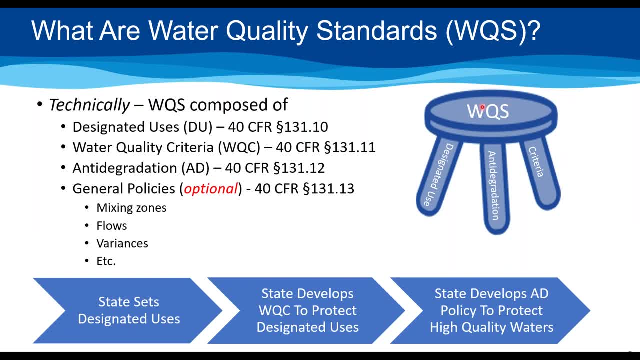 this three-legged stool. you know the way you make the water quality standards balance out is by having those designated uses criteria in an anti-degradation policy, and so if you're really curious of looking at where those are at the regulations, you have designated uses. at 40 cfr 131, 10 water quality criteria are described in. 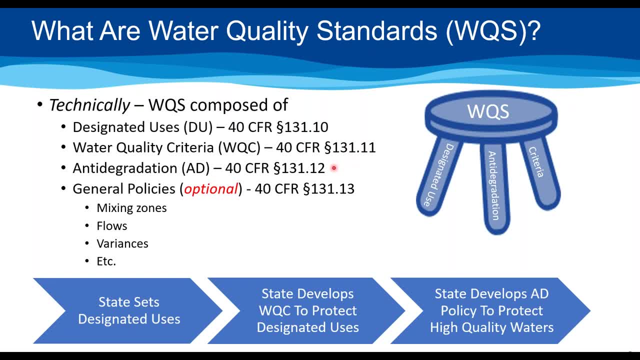 131 11 and any degradation policies in 131 12.. and then that rule also says states can optionally- they don't have to, but they can optionally have other policies in their water quality standards and you'll often see things like mixing zones of the. 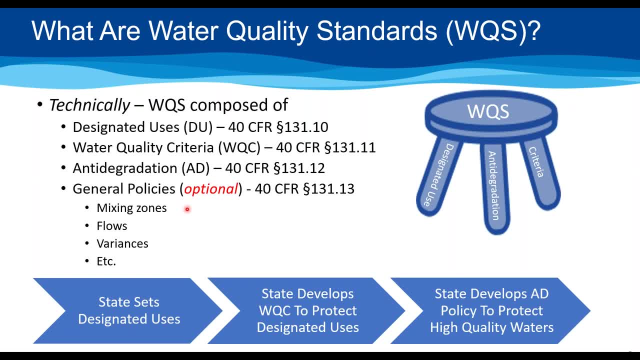 state wants to say: well, you don't get the full river, the full stream that makes your waste in, you only get a portion of it's, a mixing zone. they may discuss the flows that are used in those policies, they can discuss variances, and that's something you're really not going to get. 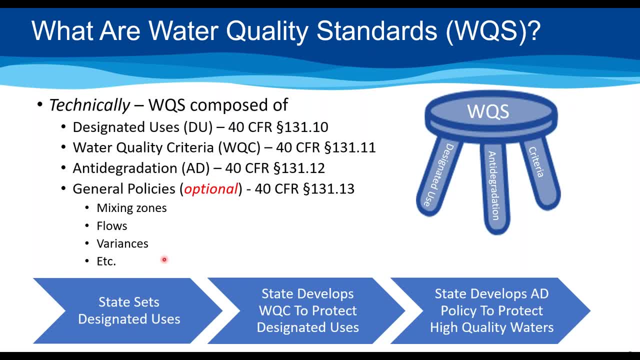 into. that would be a topic for a whole session on its own, and then there could be other policies that the state has. but the general flow of how standards work is that states set designated uses, and these are these: how do i want my water to be used? how do i want each water body to be used in my 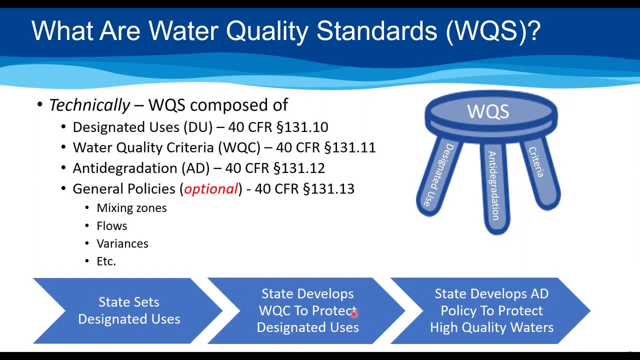 state okay, and once i identify that, i say well, okay, well, what kind of water quality criteria do i have to generate to protect that? you know, for instance, dissolved oxygen. most people would say that a warm water fish would need five milligrams per liter of dissolved oxygen to survive. 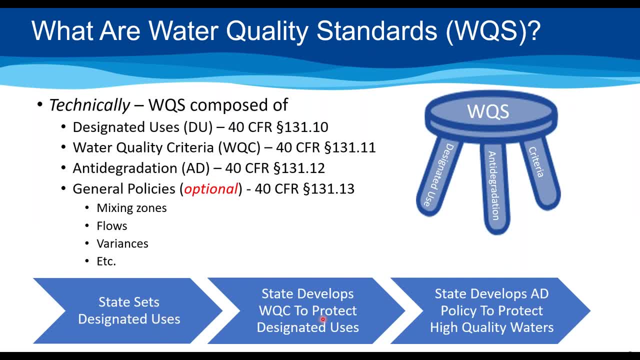 so if you have warm water fisheries designated uses, one of the criteria that you're going to have to protect that use is all toxin. and then, after that part of it's done, you know the state should develop an anti-degradation policy to protect their high quality waters. and i'll get, i'll spend quite a bit of time. 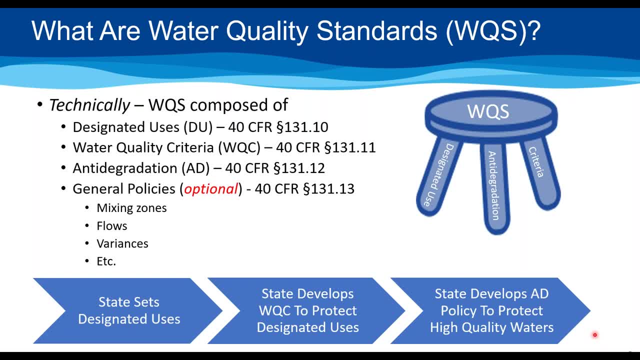 with any degradation. i think it is the least understood part of the standard which i'll get to when we we get to that part and i'll talk a little bit more about that in the next couple of weeks and then i'll try to explain to you why that is. 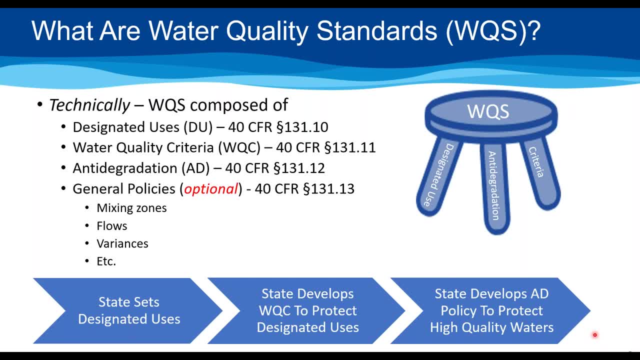 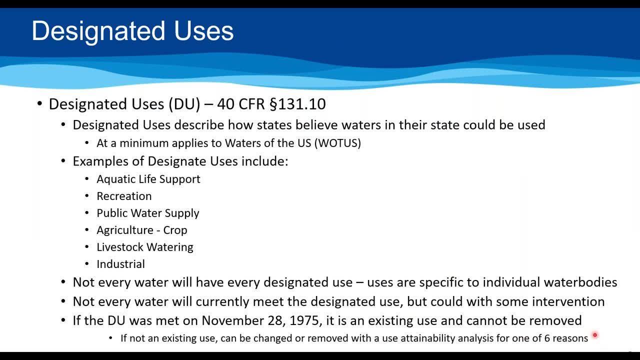 and it probably should be understood better and have a lot more impact than what i think it does. so this first part, you know, that first leg of that water quality standard stool is the designated uses. okay, and designated uses: again, they describe how a state wants to use. 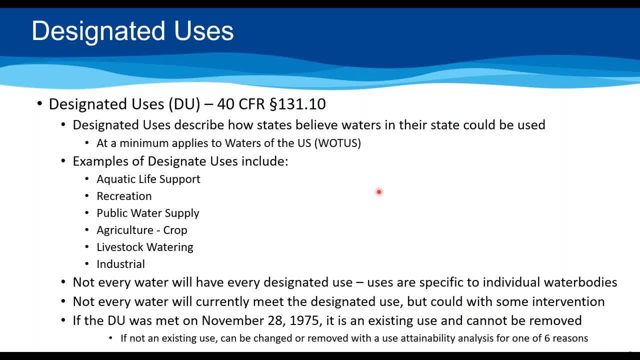 the water and at a minimum, those apply to waters of the us. you know what's been going on over the last dozen years or more. there's been a lot of back and forth over what is the water in the us. recent supreme court case ruled on that. 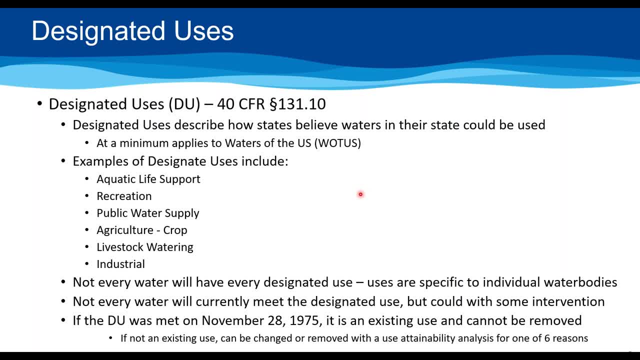 particularly applying to wetlands. i won't get into that, but i will just say they apply all the waters of the us and in some cases, if things aren't even water in the us, some states will divide waters of the state and in their water quality standards they 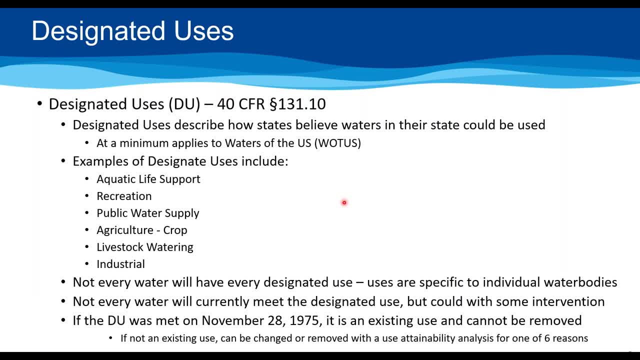 apply the waters of the state that may not be waters of the us, so designated uses, the two we often see because of that goal of the clean water act. it's aquatic life support. how do we support the aquatic life in the water? um recreation, and you saw the clean water. 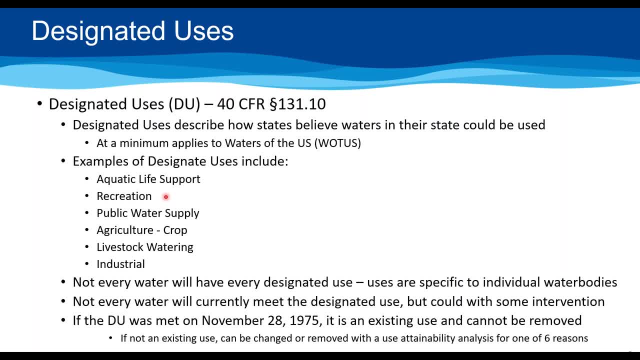 act goals recreation in and on the water. sometimes hear that referred to as contact or non-contact recreation. think of that as swimming or as the in the water and contact and perhaps fishing from a boat, boating- that type of thing is made non-contact recreation on the water. 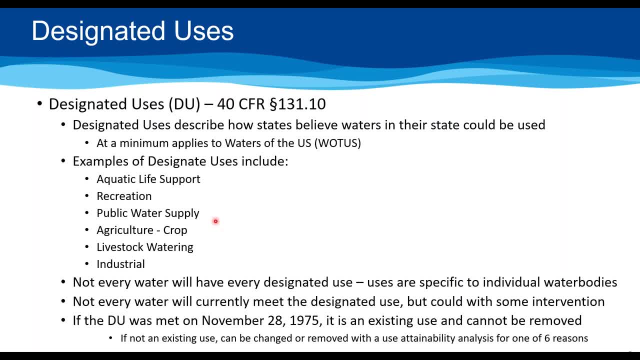 states then come up with their own designated uses. you'll often see public water supply as a designated use. i want to use that water body to perhaps drop a pipe in and pull my source water for my drinking water out of it. you can have agricultural crop use. there's some things that humans in a public water supply can. 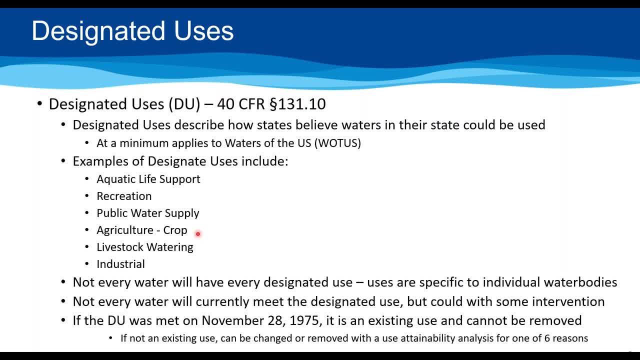 tolerate just fine that crops might not. so you may have to have a criteria, some criterion, for various things that would affect agricultural crops, livestock watering, the same thing. there's things that don't affect you and i much at all, that really could affect livestock. so you might want to have that as a use if. 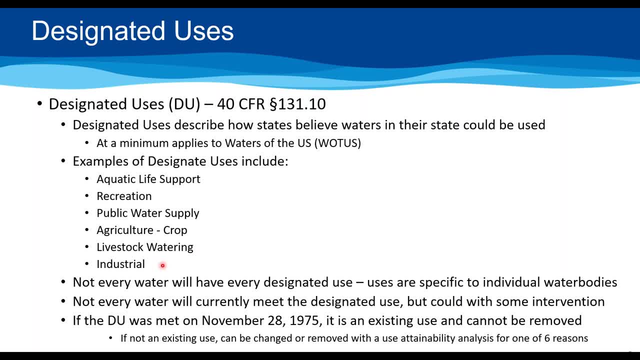 you're running a large livestock producing state industrial water uses some people might have- and, like i said, it's up to the states to do it. so there's a lot of other uses that could be out there, depending on your state and what they've adopted. but what i will say is that not every water will have every designated use. 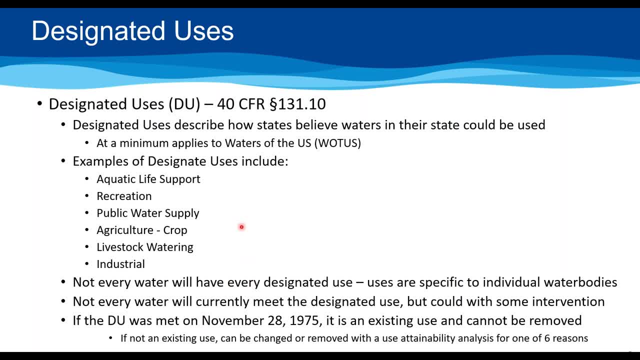 you know their specific individual water body. you may have one that only has aquatic life, support, recreation kind of things. so i'm going to go back to the past and look at the states that have a listing of water body uses and then i'm going to go back to the states that have a listing of 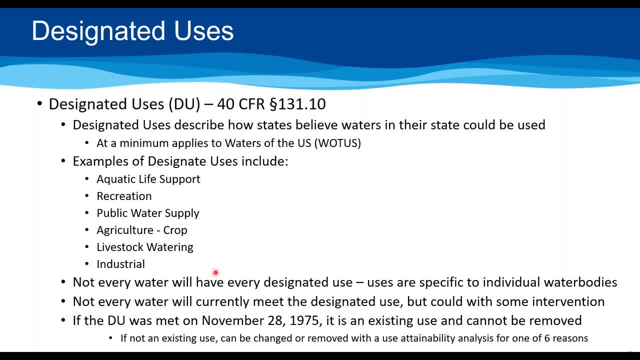 water segments, uh, you know, by stream or lake, what have you? and you'll have to look at that particular water body and look and see what uses have been designated for it. so, uh, and not only is that a, and not everybody, not every water body will currently meet its designated use. 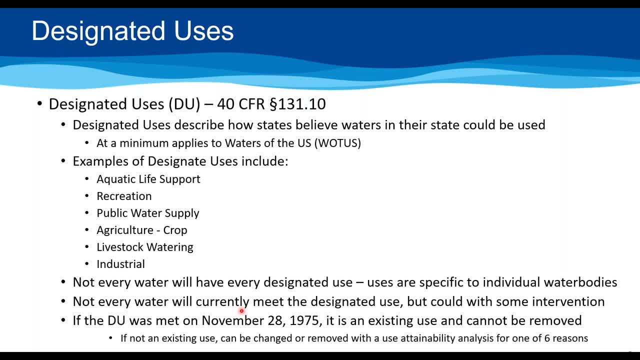 where you get these impaired waters and tmdls we'll talk about, but they could with some intervention. that intervention may be better treatment from the wastewater treatment plant. it could be non-point source control. what have you? so just because a water body doesn't meet the designated use doesn't need. 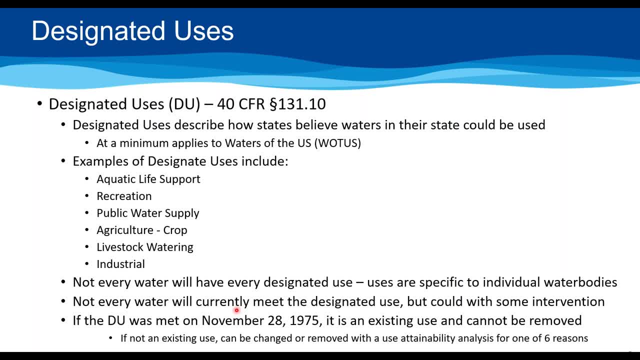 to keep still have the designated use. and then one of the really uh interesting parts of the rule is it says that if a designated use was met on november 28th of 1975 as an existing use and it cannot be removed, well, we're almost 50 years out from that. 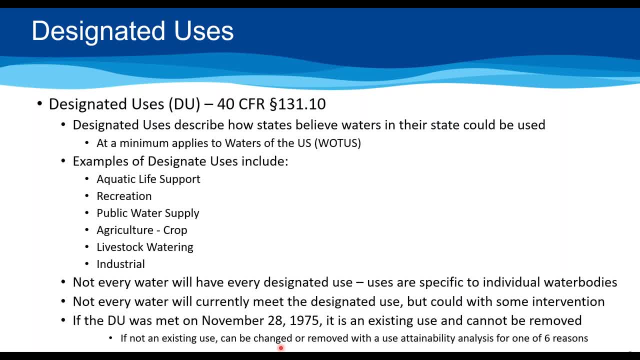 now. so it's kind of hard at this point in time to go back and figure out what may have been met in 1975. but some states have some pretty good- uh- older data where they did that. they looked at it, were able to set their uses in terms of what they believed were existing. 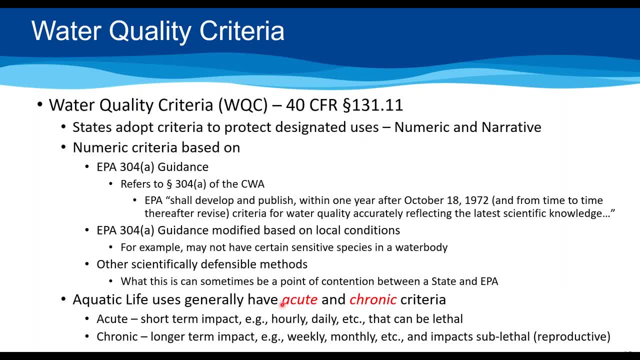 uses. okay, so that's our designated use part. that's pretty straightforward. water quality criteria. it's quite a bit more complicated, in my opinion, and you'll find that in the code of federal regulations, title 40, 131, 11.. so we'll talk about that later. but what happens there is that states adopt: 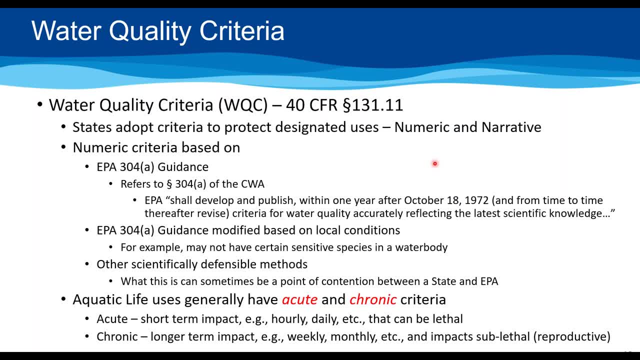 criteria to predict designated uses, and they're both numeric and narrative. uh, criteria that get developed by most states, and the numeric criteria are based really on a couple of things. uh, epa 30, what's called 304a guidance, and 304a refers to section 304a of the clean water act, said epa. 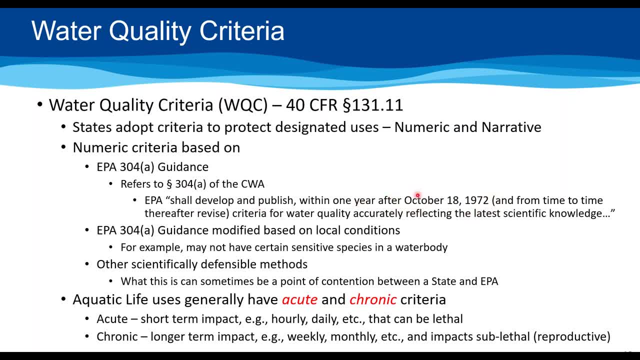 Act was published, they would publish within one year of 1972 and time to time thereafter, criteria for water quality for really the latest scientific knowledge. So you'll see, EPA will have probably have water quality criteria in development. right now Go back and look at old criteria. I think in my time, you know, in this field in the 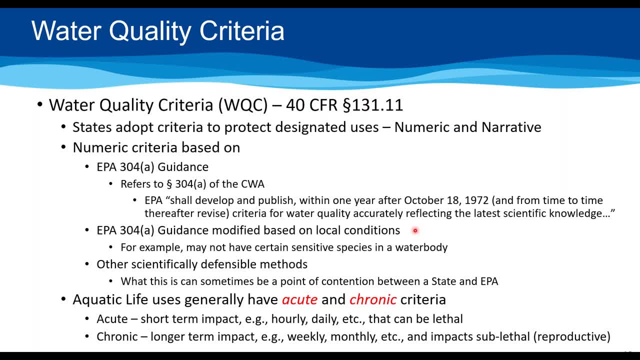 last 30-some years there have probably been four iterations of ammonia criteria to affect municipalities and their discharges. quite a bit. Those 304A guidance documents can then be can be modified based on local conditions, and one of the reasons you see from that fairly often is that the criteria developed by exposing 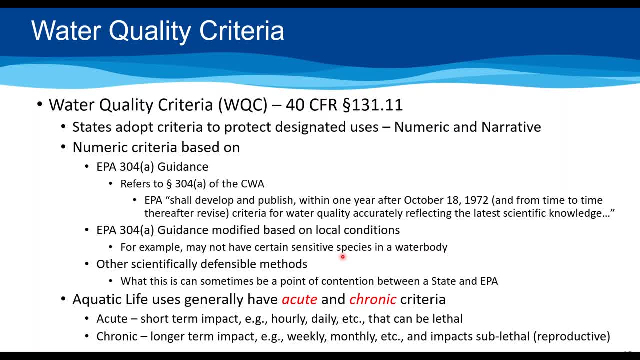 a number of species And you tend to pick the most sensitive species. Well, it may so happen, you don't have those most sensitive species in your water body, so there's a method to recalculate that. Then you can have just a general, other scientifically defensible methods, and that's sometimes. it's 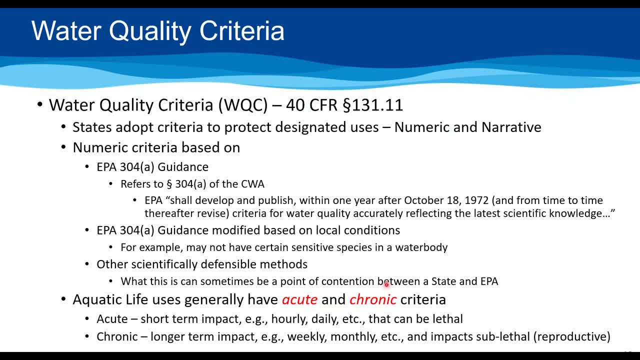 a point of contention between the state and EPA. State may feel they have a very scientifically defensible method for coming up with a criterion, but remember that EPA has the approval authority. So you know, that's a very, very important thing. 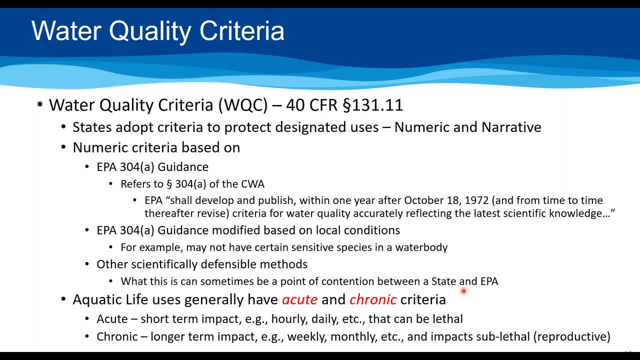 Thank you, Thank you. So we're going to go to the next slide. So we're going to talk about the second criterion. There's a couple of things that people may have in mind. First, we're going to talk about the criteria. 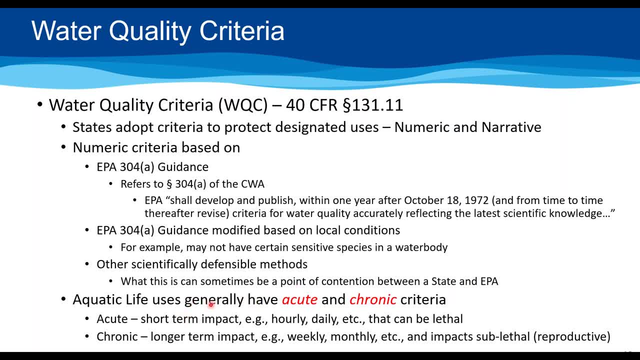 The second criterion is that they're going to have to be sure that they've got the right criteria. So they're going to have to be sure that they're going to have the correct criteria on the water quality criteria, And if they disagree then it's not going to come to pass. 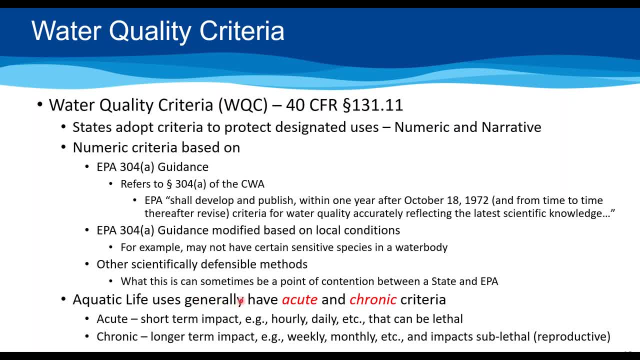 The other thing to remember then, particularly on this aquatic life criteria, which generally dominates a lot of permitting actions that people are exposed to out. there will have acute and chronic criteria, So within those criteria, same polluting, you may have two different values being just. 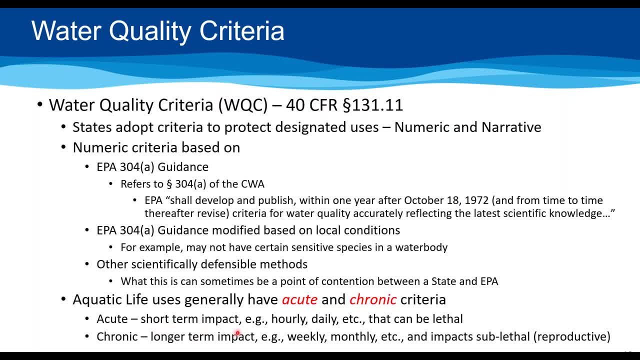 for a refresher. and acute is a short-term impact, hourly daily, hourly daily, something that could be lethal and by that means it can kill sensitive organisms. Chronic is a longer term impact and that tends to be a weekly or monthly impact, and 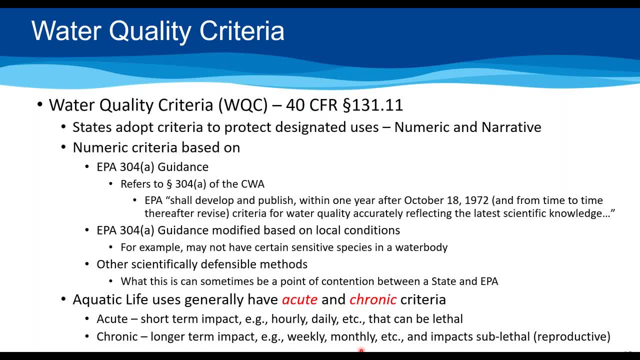 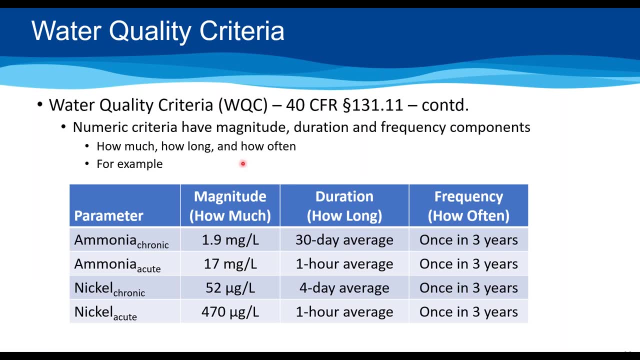 it has what are called sublethal effects, that we call reproductive say that organisms will produce as many offspring as they would if they weren't impacted, or the offspring may be stunted Within those water quality criteria. then they need to have what are called magnitude. 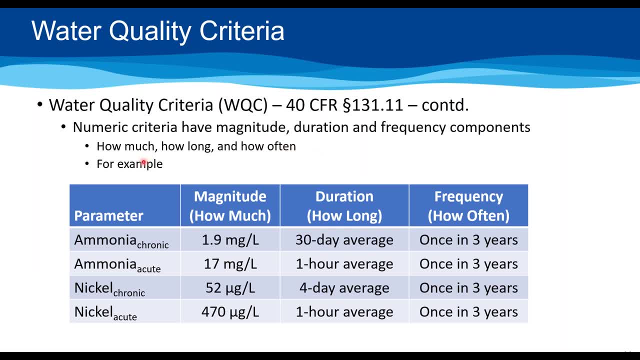 duration and frequency components, and you can think of that as how much of a pollutant makes effect, how long can an organism be exposed to it and how often can it be exposed to it. And I'll just give you an example here of these top two. of ammonia, you've got the chronic. 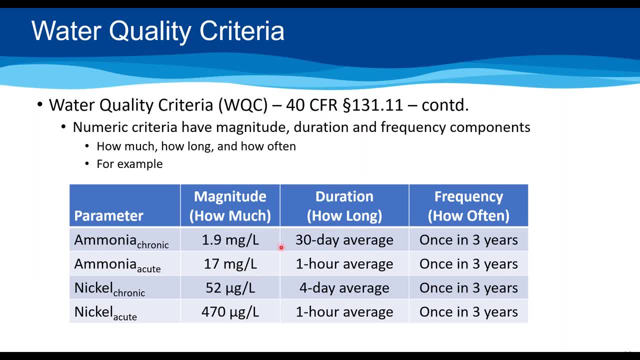 and the acute criteria here. And so it says over: you know you can have 1.9 milligrams per liter over a 30-day average. so magnitude, duration, and then how often can that happen? once every three years. 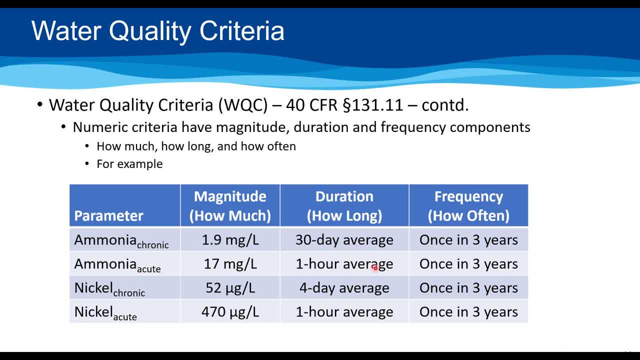 The acute, which, remember, is a short-term duration and in this case a one-hour duration. the way the criteria are set up, It's going to be a lot longer, It's going to be a lot higher because that short-term exposure, you know, for lethality. 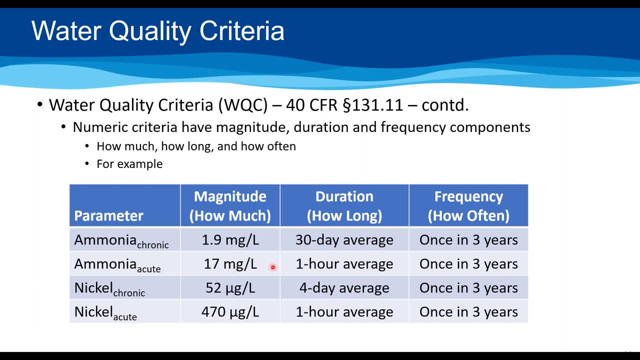 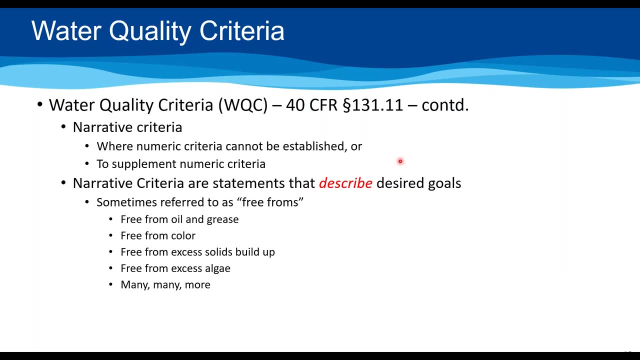 actually killing the organisms can be quite a bit higher, but it's magnitude: 17 milligrams per liter with a duration of one hour and a frequency of one to three years. Then you have what are called narrative criteria. you develop narrative criteria where numeric 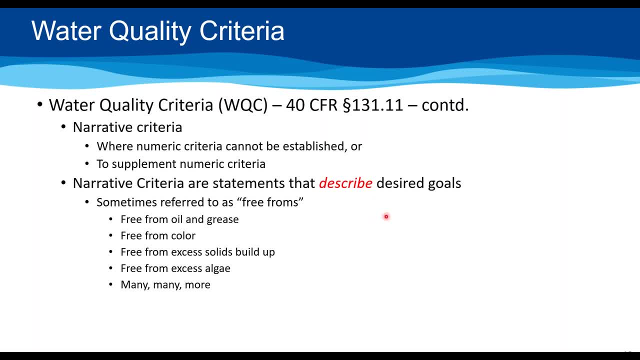 criteria can't be established Or you want to set a standard. You want to make sure you're following all the criteria and then you can supplement the numeric criteria. Narrative criteria often describe the desired goals for water and people refer to them. 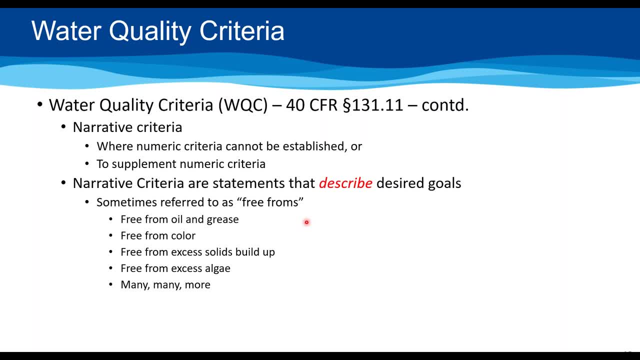 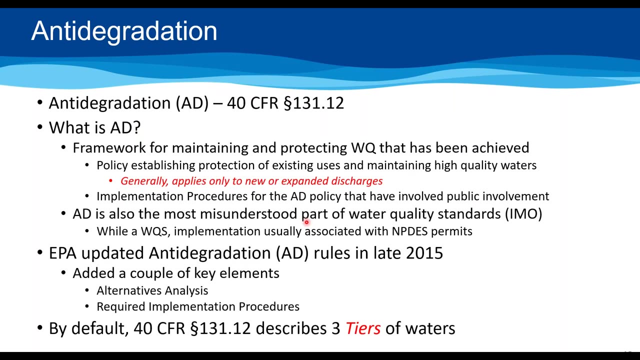 Sometimes it's the free froms: free from oil and grease, color solids, build-up, excessive algae and lots of whatever essentially a state has come up with. So those are the first two legs of the stool. The last two legs are, you know, the one I told you that I think is the least effective. 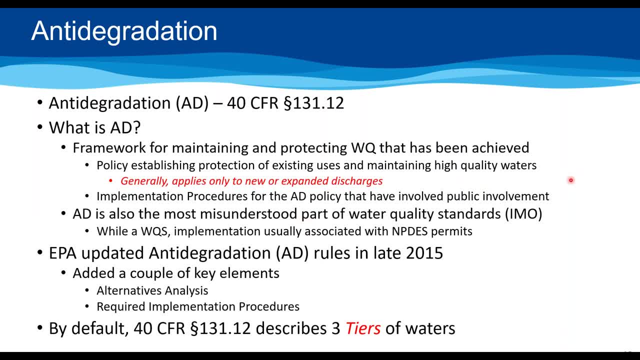 and that's a little bit more soil-based. It's a little bit more soil-based and it's not the most effective, but it's a little bit more soil-based and a little bit more soil-based, least understood, and it's an anti-degradation. An anti-degradation is what's called a framework for 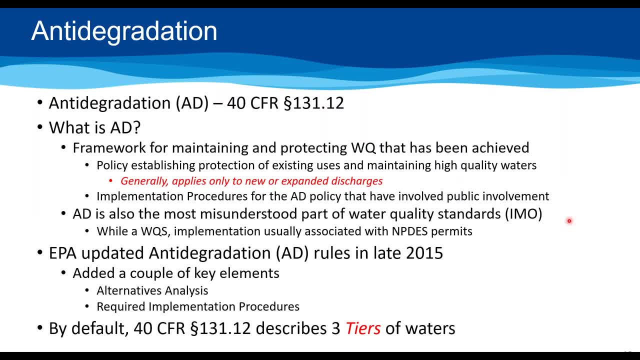 maintaining and protecting water quality that's been achieved. So if you meet the criteria you've established for your designated use, let's try to keep it there. okay, Let's not let it get worse. and if it's even better than it needs to be, let's try to keep it better than it needs to be. 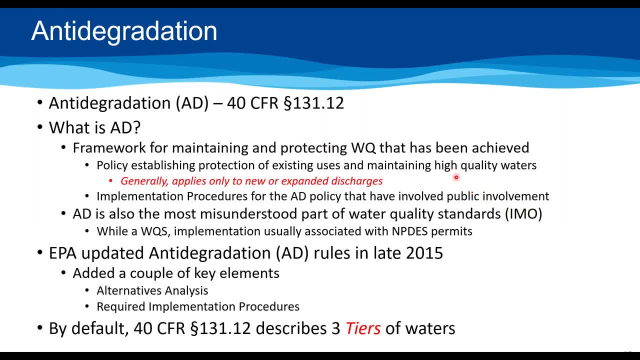 if at all possible. That's kind of what anti-degradation is saying. It's a policy that generally only applies to new or expanded wastewater dischargers. So if you're getting a permit renewed, you can only see that It's just if you're expanding your discharge or if you're 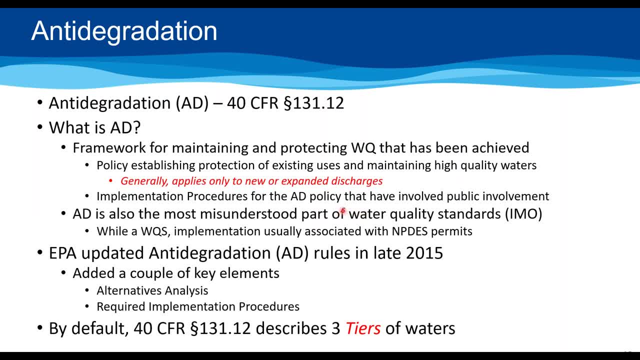 a new discharger, you'll often fall into the anti-degradation policy of the state. It involves public involvement, So know that, just like your permits put out on public notice, if a state makes a determination on any degradation and allows you to initially degrade some high quality. 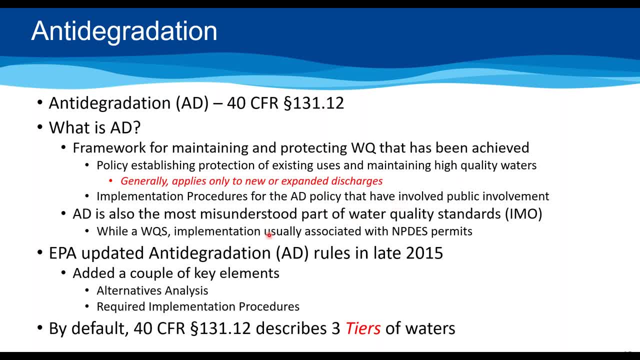 waters. they have to put that out for public comment and involvement also. So, as I said, I think it's most misunderstood. I think a lot of that is because it is a water quality standard, but implementation usually gets associated with NPDES permits, And so do the permitting people. 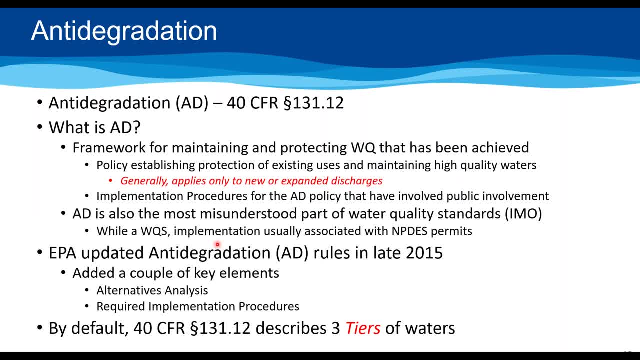 have the same understanding. Yeah, I think it's more of a understanding of anti-degradation as, say, the water quality standards, people, And sometimes there's a break between those two groups and their different understandings of how that applies. But EPA made some good updates to the anti-degradation rule in late 2015 and added a couple of really key elements. 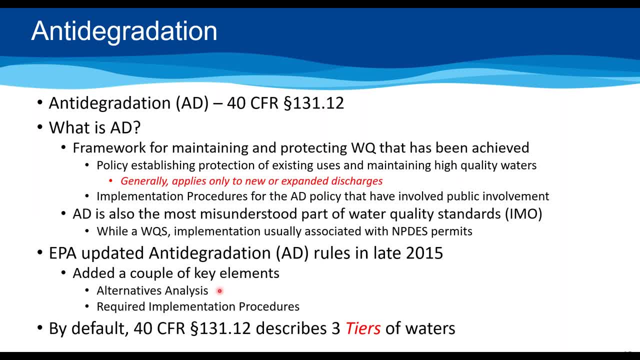 One of those is an alternatives analysis, which says that if you're one of these new or expanded states and you have proposed a discharge and you have what's called the base case condition, where you can just pull it up to the maximum, you should look, you know, if you're in one of these. 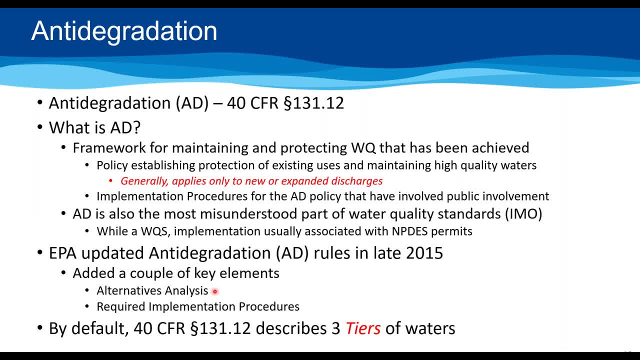 high quality waters at alternatives, And if you can essentially afford to do the alternative, you should do it to keep the water at a higher quality level. It also required that states develop procedures that involve the public And, by default, that this anti-degradation in the federal regulations defines three tiers of waters. 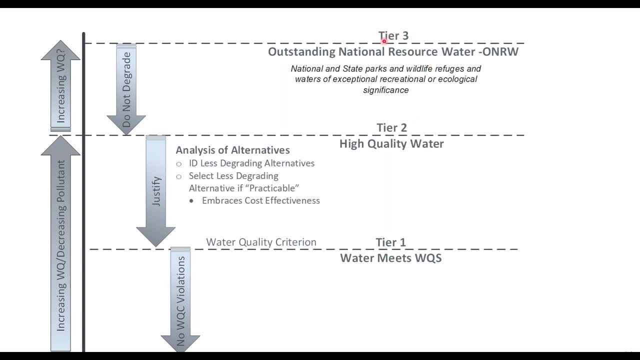 So I like pictures. So these three tiers of water are called. tier three is outstanding national resources, O&RWs, and those can be national parks, wildlife, mayonnaise, a standard water source, And then, in addition to that顽 is the most important. January on the first five years is the quite a U降 water resource And they were Secretという brush, So it's really early on this year this five year status question for us Again. at least 5,000 in 2017, 서로 swapped communities for over one year And it's really Bear Point. 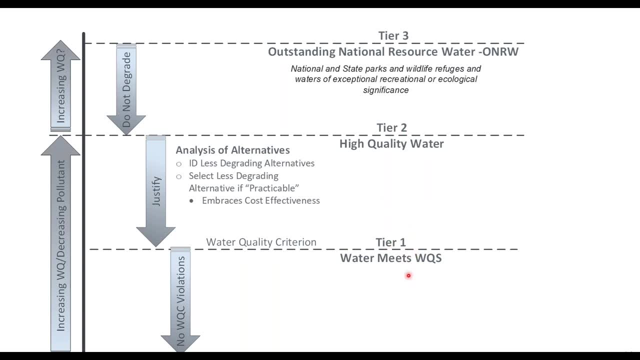 You have a lot of opportunity for you to think about this and plan some decisions when you're kind of at this point, And then the utility and other items in this slide on your before and after. kind of interesting about this Most of the time the information you see they want to. 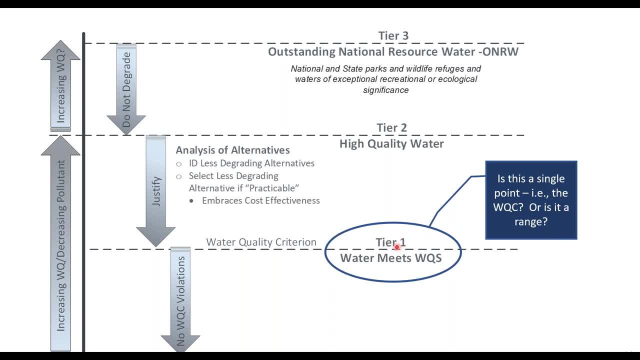 treat Tier 1 like it's a single point, like just meet the water quality criteria. I think probably it should be looked at more of a range, like maybe 10% either side of that, something to think of that more as a range because you know water bodies are going to. 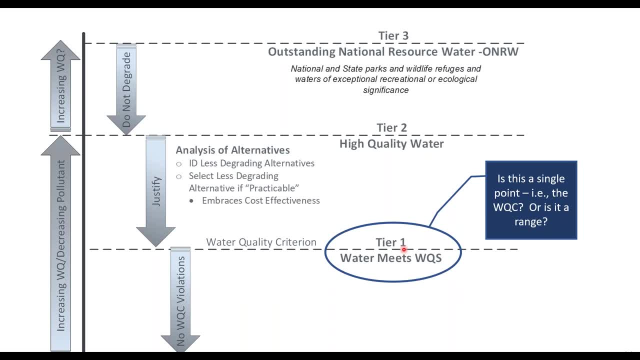 flow at different levels. They're going to be exposed to different things different times of year, And it's just. it's really hard to say: boy, I just came right up to that standard and that's it, And so I'm at Tier 1. So it's a little hard to describe. 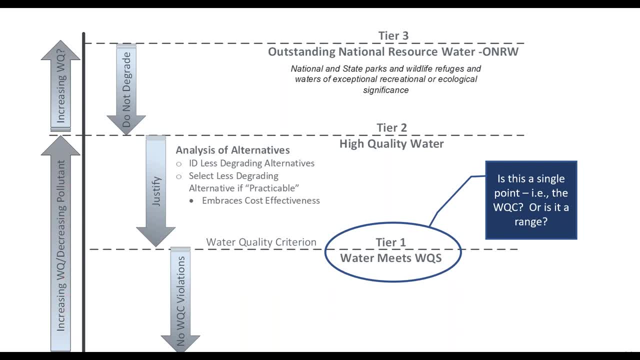 So what I want you to see over here is that you know well, okay, well, that sounds logical. Tier 1,, Tier 2, you'd be increasing water quality, So you want to decrease the level of pollution. That makes sense. And so you think, boy, these Tier 3 waters must have really. 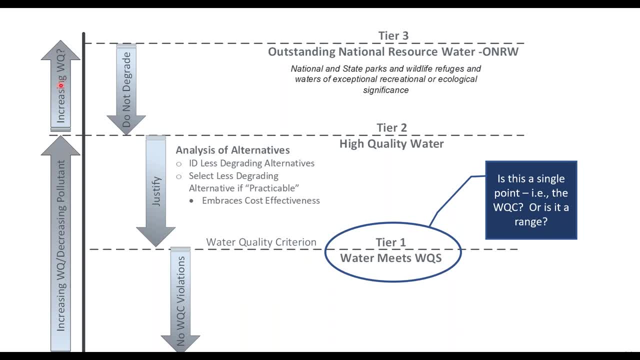 super high water quality. That's not always the case. In fact, in Kansas, some of the only ones we have really fall into this kind of ecological significance. The one I give you an example of to make a point is what's called the Quivira salt marsh, So salty water. 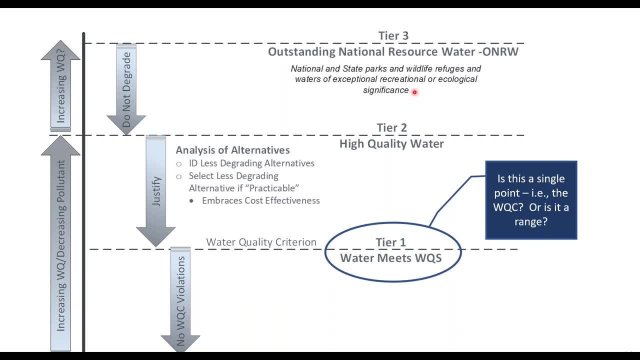 Awful. You'd never want it for drinking. You really wouldn't want to recreate in it. Not a very good quality water. but it's of great ecological significance because it's a place where migrating birds from Canada going south migrate to every year And they're very unique. So it's something you would want to protect. And so what happens? 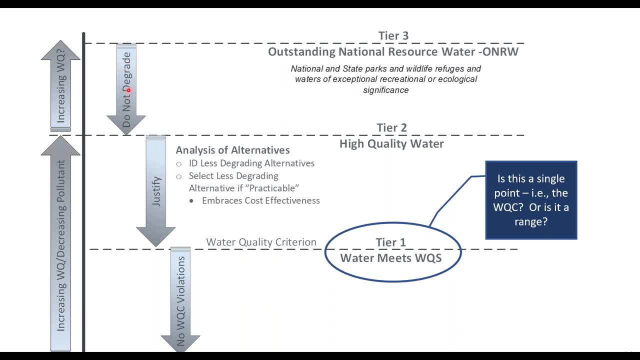 if you want to protect that, Well, you say I'm not going to allow any degradation to happen in a Tier 1 water. So I'm not going to essentially allow any discharge, Because if anybody can discharge something that has absolutely no impact, I'd be surprised. 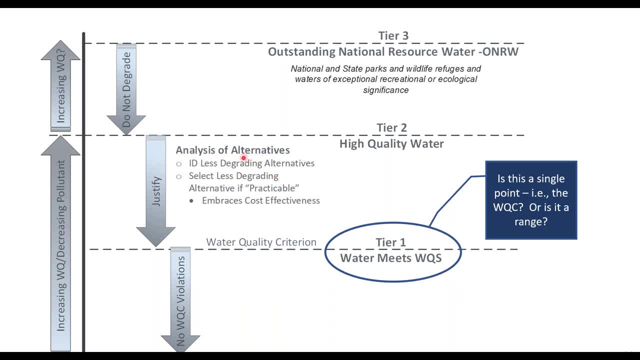 So in these high quality waters- this is where you do this analysis of alternatives I talked about- You identify less degrading alternatives, You select one that's practical, And that term practical kind of embraces the thought of cost-effectiveness. So you have to justify. 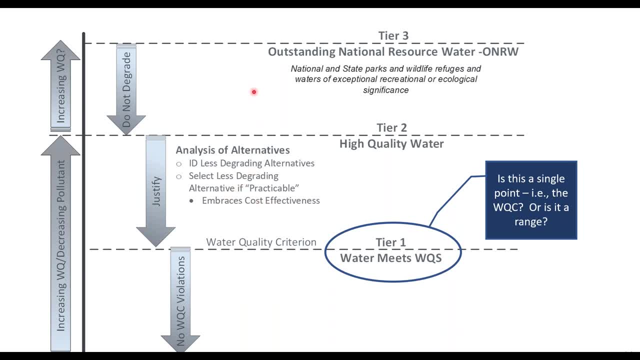 why you would want to discharge. Well, what happens in practicality is that states begin to catch on. that you know, if I make a water at Tier 3 water, I better hope I don't want anything to ever discharge. and Because I say it can't allow any degradation And that's a pretty tough standard. 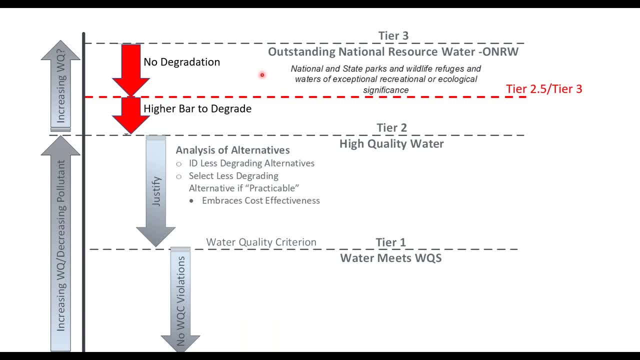 to put on people is to basically say no discharge, to be, you know, careful. that would happen. and so what a lot of states have done with epa approval- although it's not in the regulations- created what's called a tier two and a half water. 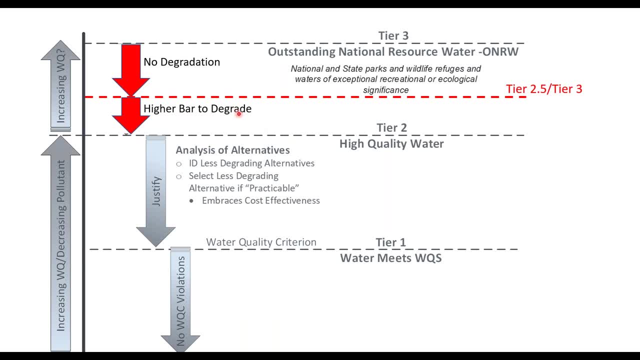 and a tier two and a half water essentially could be degraded, but it's got a much higher bar that the discharger has to beat, as opposed to a tier two water, before they would be allowed to uh, degrade that water by. so that's kind of the practical assessment. there are some states who 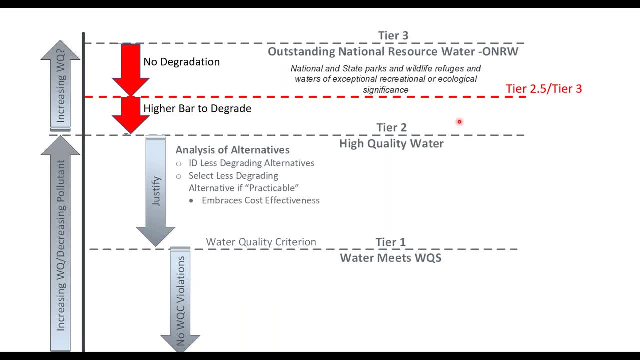 made tier three waters they wish they hadn't, uh, and a lot of them caught on pretty quick. i don't think you'll find many tier three waters out there. you can look in state standards and i've seen a number of states who have none, zero tier three waters, uh, whereas, like i say, kansas, we did. 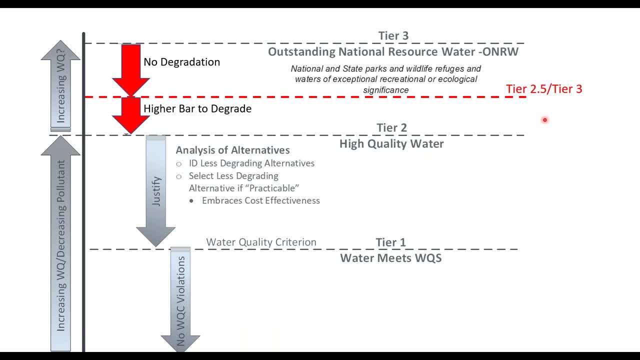 try to identify those that were really, you know, exceptional significance and that we really would never want anybody to discharge into. and again, a practical example i give you. that is in kansas there's a lot of most lands held privately and so there's very little access to a lot of water bodies, but you have a few big rivers in. 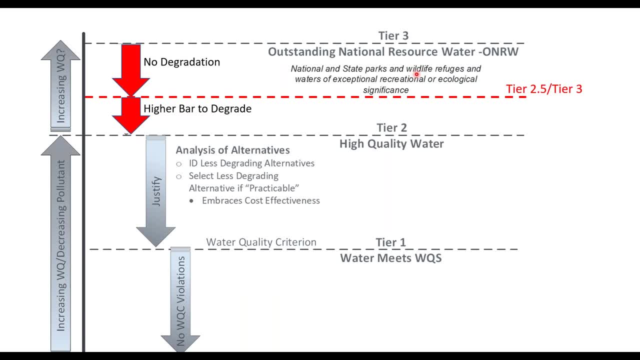 the state, like the kansas river, that do allow recreation, and so at one point a group of canoeists and kayakers wanted kansas to make the kansas river in a oh in rw tier three, because they said: well, that's exceptional recreational significance, there are many more life in the state and that seems to 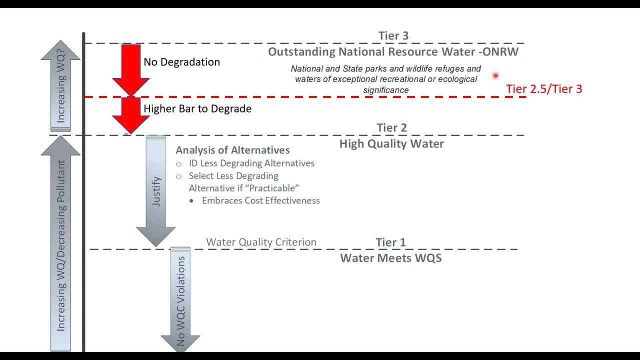 make sense, and until you think that kansas is a state with a little less than three million population and a million of them live along the kansas river and so there's always going to be some kind of growth, there's probably all going to always going to be some kind of new discharge, etc. 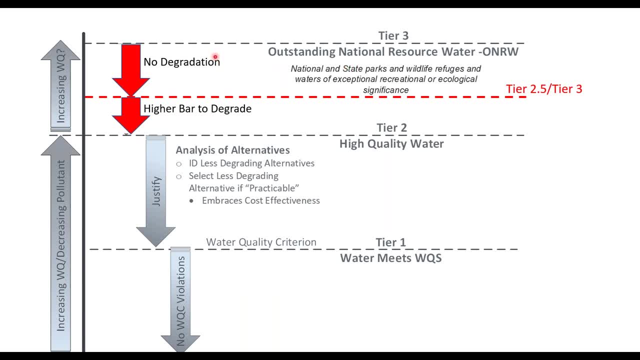 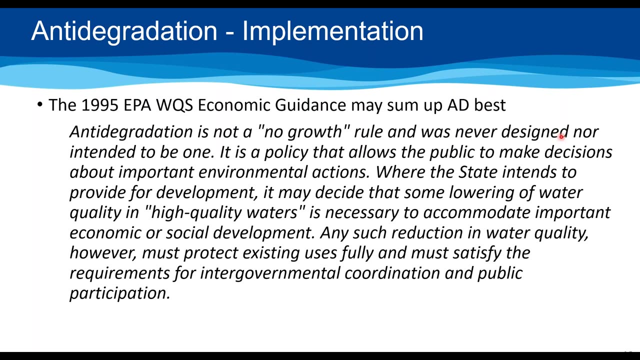 so it would be really difficult to say, oh, we're going to make that tier three and never allow any degradation again. and so it happens to be one of these tier two and a half waters in kansas which does allow some degradation but makes it a very high bar to achieve that. and, as the epa 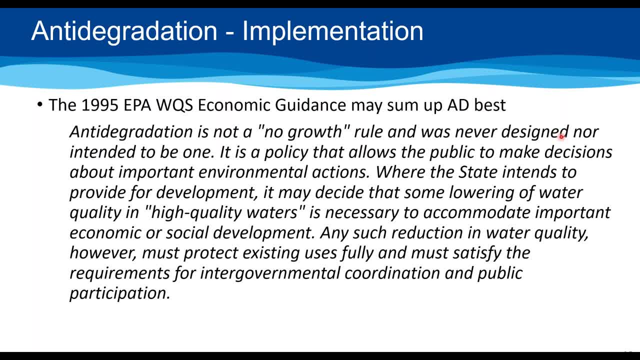 has said in their guidance documents that any degradation is not supposed to be a no growth rule, although i would argue that tier three waters are pretty much no growth. so same thing with the keystone river, where you come in and you see the delta zero being they seem to have a little bit of no growth, and so i think it's a good way to just sort of 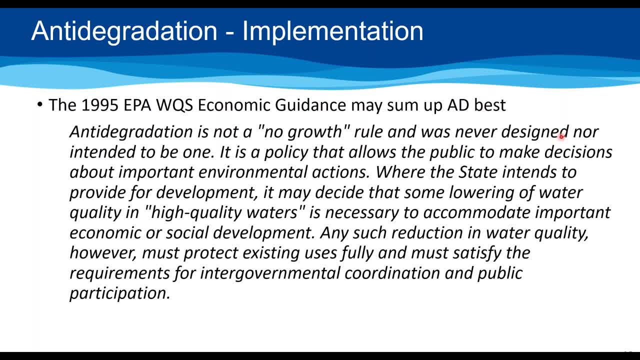 sort of put it right so it's a good idea to do that right is not challenging the use of that. i think the other point was that kansas is just designed to let the public have a say if the state wants to allow an area to develop and there's important uh reasons socially or economically for allowing that and allowing a lowering of water quality. that can be done, but you have to go to the public and you have to notice it. you have to tell them if they want to challenge that, it can be challenged and it may not be allowed. so that's really what any digger did on the top there, just want to一. 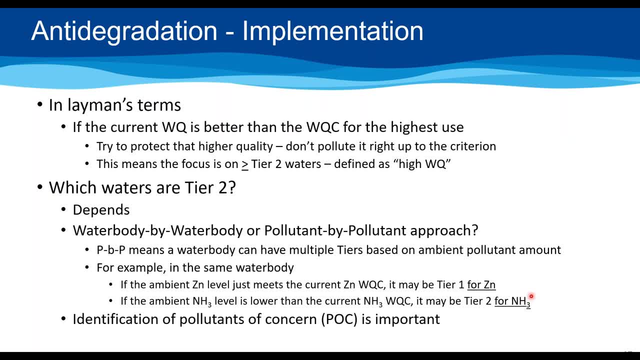 I'd say in layman's terms: if current water quality is better than the water quality criterion required for the highest use, you try to protect it. You just don't follow the criteria. So most of the focus, most of the action in anti-degradation is in these Tier 2 waters. 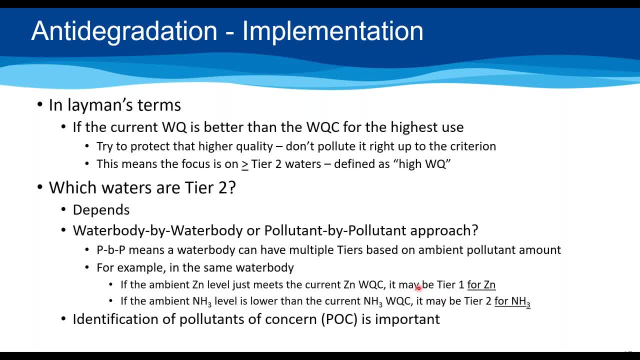 that are defined as high water quality, And so you might ask: well, what is a Tier 2 water quality? Unfortunately, the answer is that depends. You can't find it written down too often and EPA says: you know, look at a water body by. 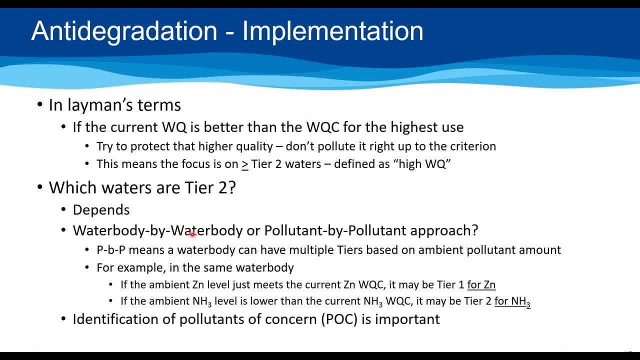 water body or pollutant by pollutant approach- Water body by water body is great. if you can do it and you've identified, you can say this river or this stream is Tier 2 or Tier 1, et cetera. Well, I'm aware of about two states who have that water body by water body approach. 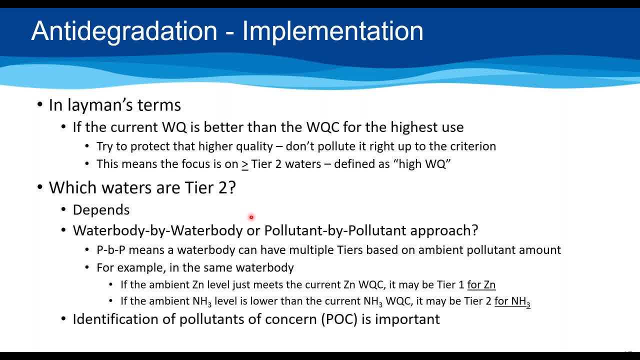 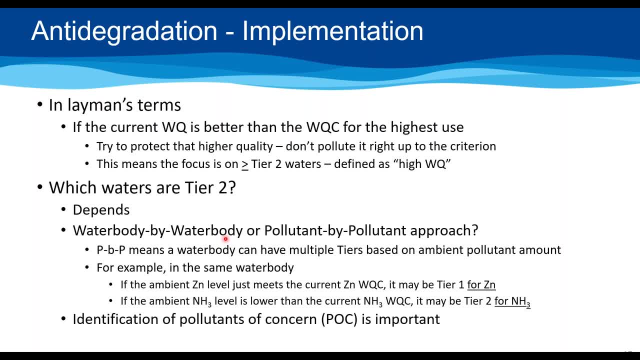 at a group of parameters in a water body and if they met it and exceeded it or exceeded it in terms of high quality, they were made Tier 2 water bodies. If they didn't, they were Tier 1, but what most states do, and what's common now, is to 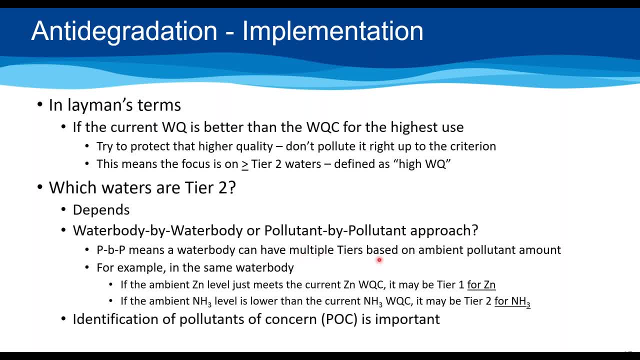 say: well, we have a set of parameters in place to replace water bodies and we don't have to replace water bodies, we can replace them easily. We can use water bodies to increase quality, and the reason for that is to use them to. 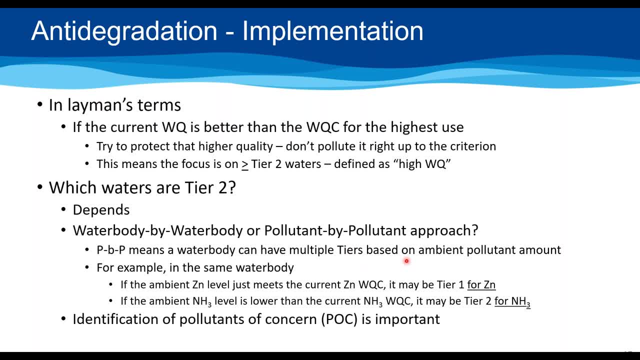 reduce the pollution, to use them as a source of pollution to have a deeper impact on our water bodies, to have a deeper impact on the air quality of the water bodies, And there's no other way that you can do that. That's the idea. 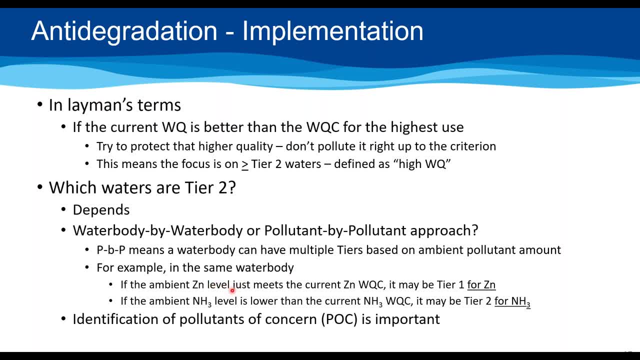 That's the key to getting this. What are you saying? that water bodies are not Tier 1, Tier 2, or are they Tier 1,, Tier 1, Tier 2, Tier 2 or Tier 5, or Tier 6, but there's no limit to what they're doing and 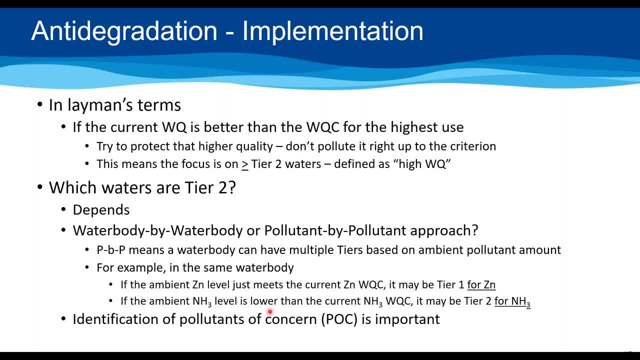 how far apart they are from what's available in them, And the reason for that is to make sure that the water body doesn't die out in the water body, water quality for ammonia and the ammonia is lower than the current water quality criteria and it could be tier two for ammonia. 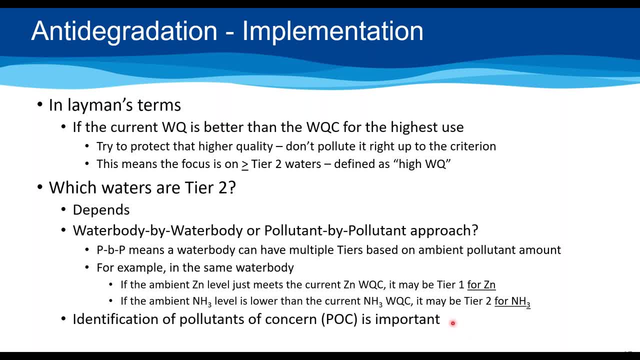 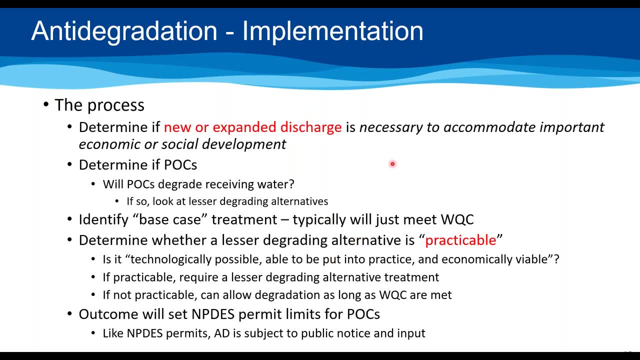 So I guess really important in these anti-degradation analysis is identifying these pollutants of concern. When I identify the ones that may be degrading in the water body and those are the ones you look to see if they're tier two, if there's an alternate treatment. 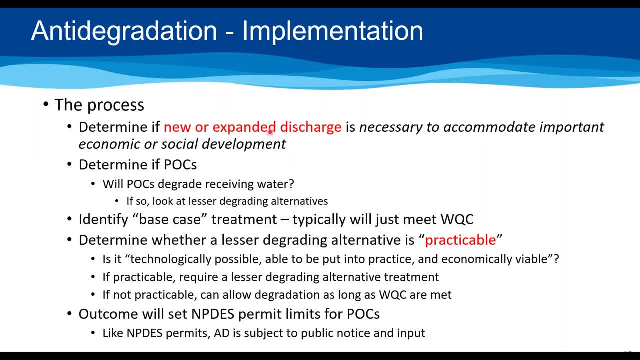 that can improve water quality. So the process that's involved is you determine if there's a new or expanded discharge and if that new or expanded discharge is necessary to accommodate important social or economic development, And if you can first make that showing, then you can proceed on to this analysis. 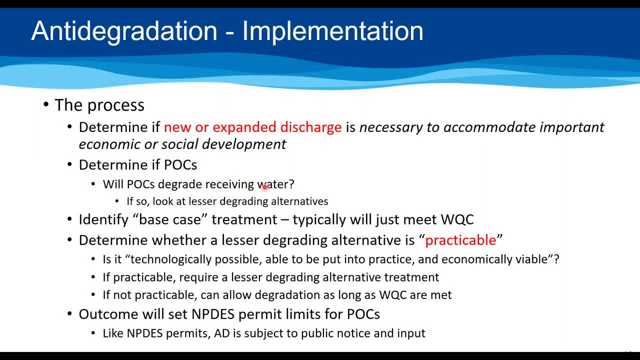 of determining what the pollutants of concern are. If there are pollutants of concern that are tier two water body, you look for the lesser degrading alternatives. So you first got to identify kind of the base case of treatment and that's typically what states do. 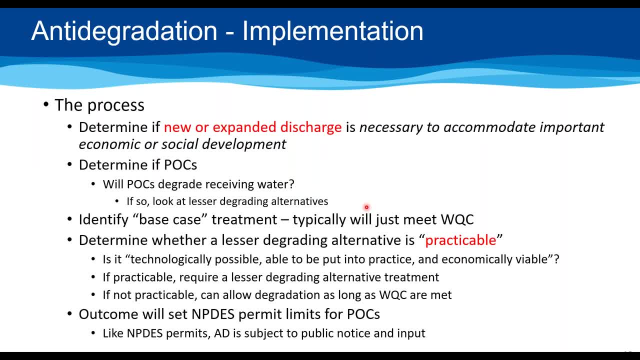 is they permit right up to do the calculations. that would, excuse me, lead right up to the water quality criteria, and that's the base case If you meet the water quality criteria, but GP just added, and so you determine whether there's lesser degrading alternatives. 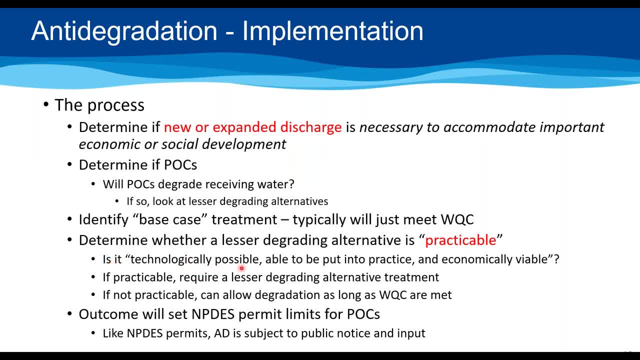 that are practical, practicable and provide, as technologically possible, able to put into practice. next, And then the last part of that is economically viable. So let's break those down. Technologically possible, is there a treatment process that could better treat the wastewater? 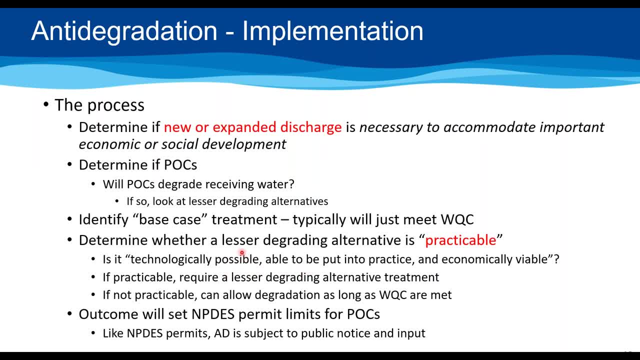 Is it able to be put into practice, And I always think of that in terms of, yeah, there may be some bench scale thing that's technologically possible. that's never been put into practice full scale, So that would not fall into this practicability. 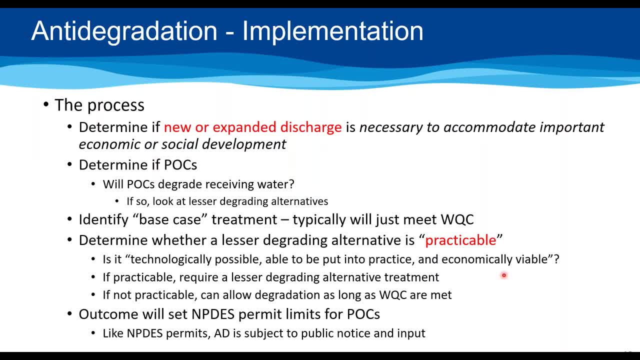 And then the last part of that is the economic viability. And that gets a lot into what I said before was kind of the cost effective analysis of additional treatment. And so what happens? if it's practical, you choose a lesser degrading alternative. 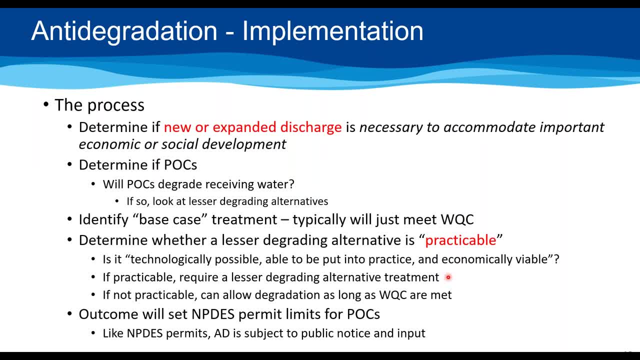 You may have two or three, four, however many you look at and you choose one of those lesser degrading alternatives. If you find there are no practical alternatives, then the state can allow degradation to occur as long as the water quality criteria is met. 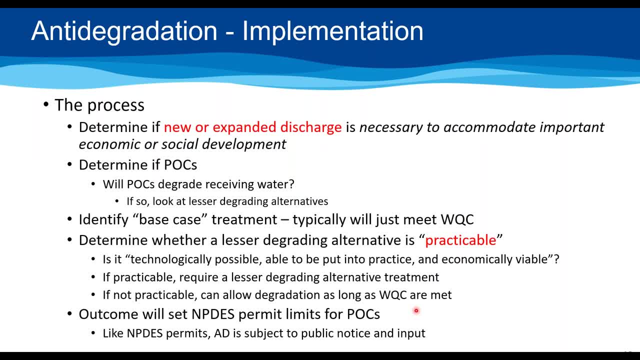 You can't ever just say, oh well, okay, well, we'll just go above the water quality criteria. And there were sounded like a lot of state regulators on the call and I'm going to bet most of them have experienced at some point in their careers. 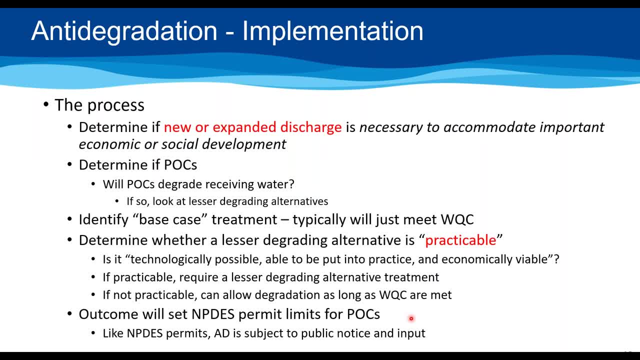 somebody going: oh, can't you just give me a number? you know that'll still exceed that, but be okay, Can you give me the authority for that? And the answer to that's: well, I'm not going to give you the authority. 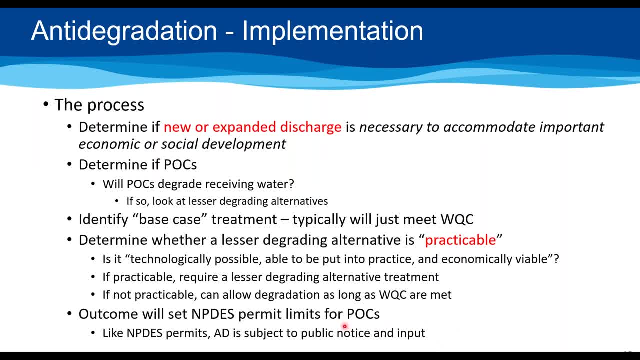 So the outcome of that anti-degradation analysis and what you look at for those pollutants of concern, concern will ultimately set permit limits for that particular parameter And, as I've said multiple times, like the permit, that anti-degradation analysis is subject to public review. 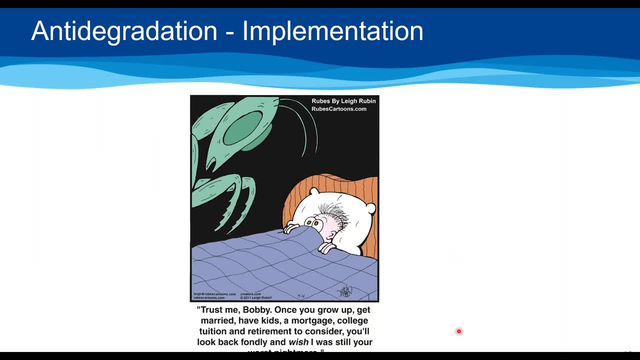 And so my wife gets me this desk calendar every year that I love. it's a cartoon called Rooms And I saw this one about you know, Bobby? you know the way that you're married and have kids and go to college. 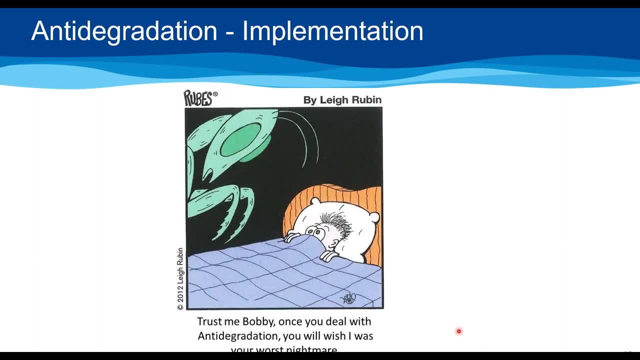 and you'll think I'm your worst nightmare. Well, I look at it like: trust me, Bobby, once you deal with anti-degradation you'll wish I was your worst nightmare. It's a real jungle to work through And in fact I did some work as a consultant now. 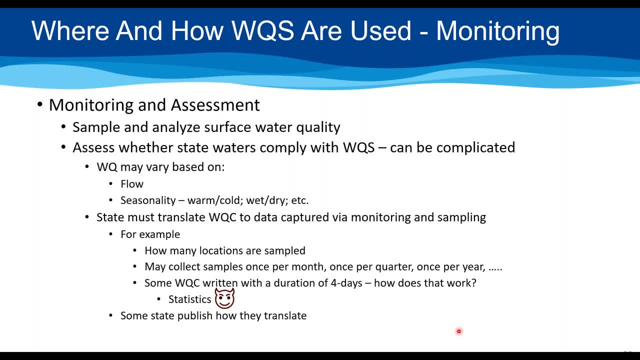 and I'm working with one that's pretty tangled up at the time being, but we're working on improving it. So that's anti-degradation. Now let's talk about how water quality standards are used. Okay, and the first one we talked about was monitoring. 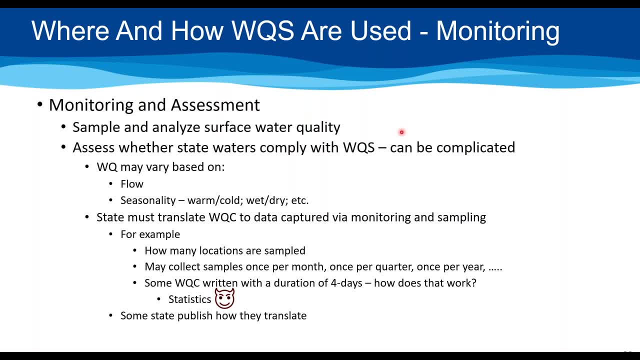 monitoring and assessment, And that's how you sample and analyze surface water quality. States have to assess whether their water quality, whether their waters, comply with water quality standards, particularly the criterion, and that can be complicated. And why is that complicated? Well, water quality can vary based on the flow. 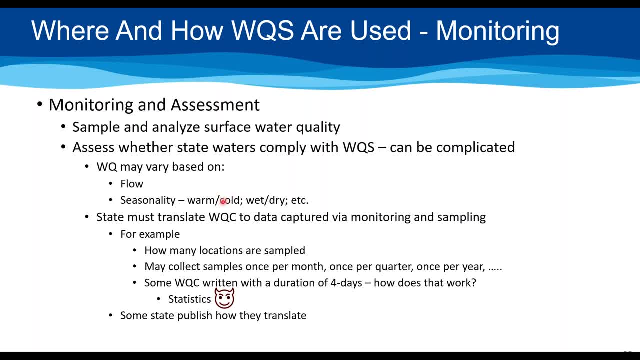 in a water body. It can be affected by seasonality- warm, cold, wet and dry. You might have leaf fall in a stream or a river fall and those can impact dissolved oxygen and color and all kinds of things that happen. 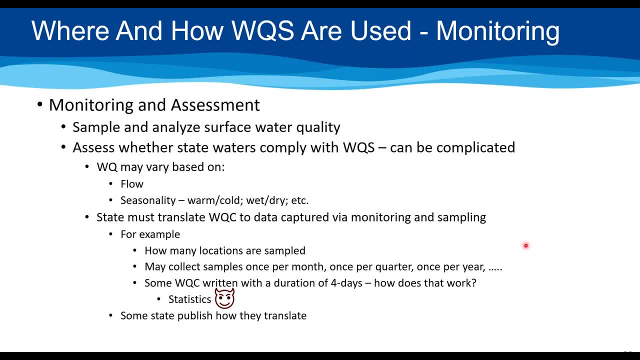 So a state has to figure out how they're going to translate those water quality criteria into the data that they capture in their monitoring and sampling, And they got to think about how many locations are they going to sample? How many are you going to collect? 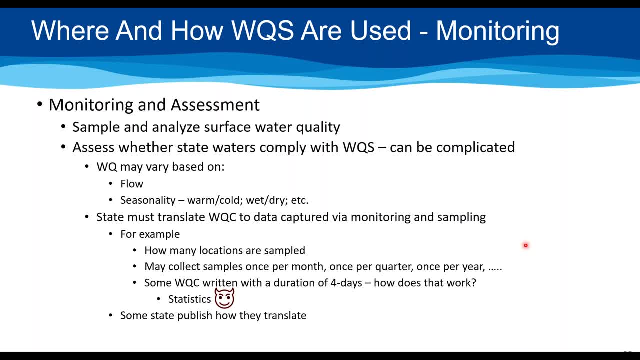 Once a month, once a year, once per year. You know, if you have hundreds of sites, it's pretty hard to do it every day and maybe even hard to do it every month. And so the water quality criterion, you know. 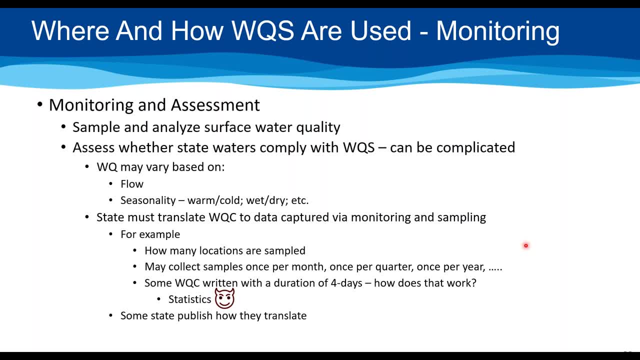 some of them are also written with a duration of four days. How does that work? You're surely not going to be out sampling every four days on that. and that's where I say: you know statistics with. you know. the devil is in the details on that. unfortunately, some states will publish those. 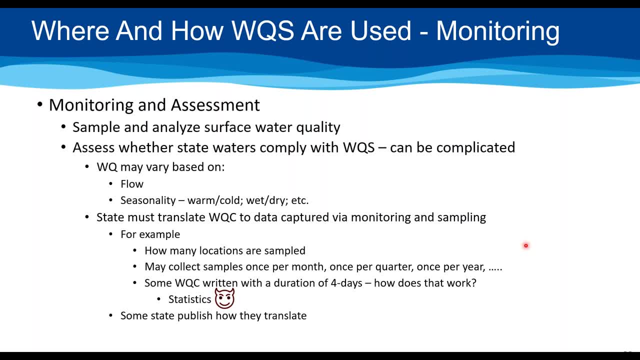 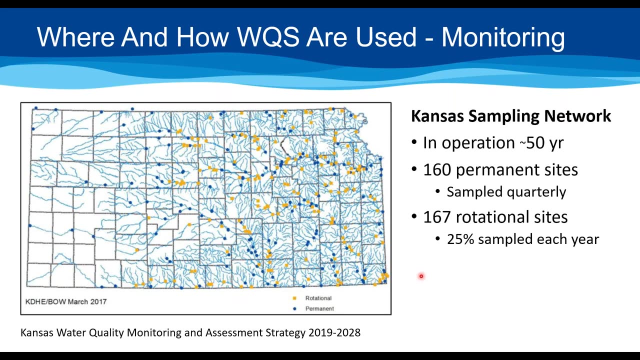 details as to how they translate the data they collect from a network into how they comply with the state's water quality standards. just to give you an example of canvas has always been kind of recognized as having a very good sampling program for water quality across the state. it's 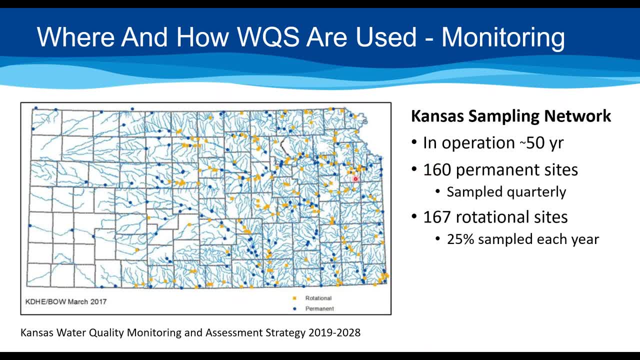 been in operation for over 50 years, 160 permanent sites, which are the blue dots, and 167 are called rotational sites, which are yellow dots. and even with those permanent sites they're sampled quarterly. okay, so four times a year is what those are getting sampled. and you look at some of these. 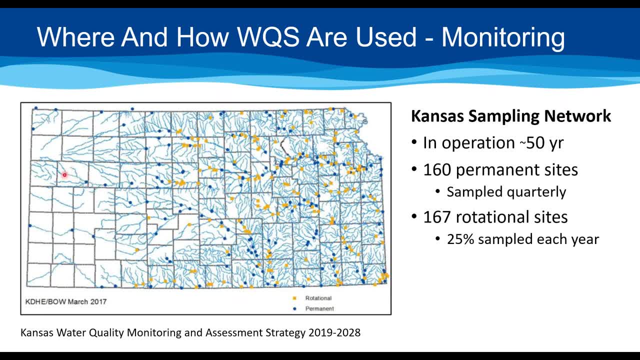 you have a station here that it's going to be determining what the state believes the water quality is for all of those upstream waters. a lot of times you'll get more dense, particularly where you have some larger cities and dischargers. but it's just to show you that in a big state you know. 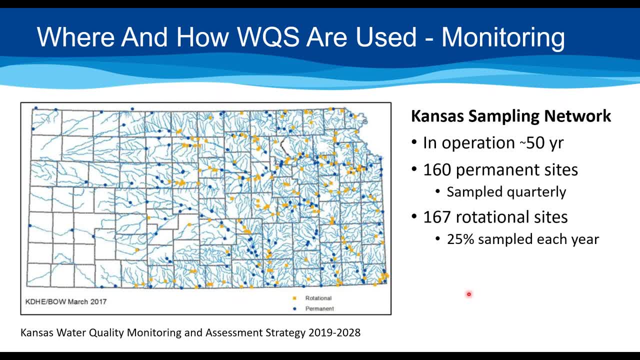 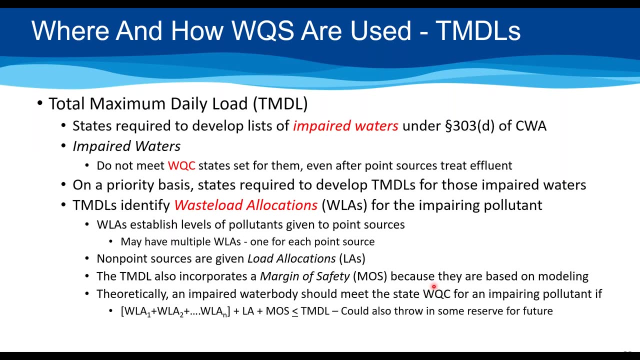 it's going to be hard to get to every water body and do it, so you have to make some calls, you have to use statistics, you have to use some water bodies that are similar to one another. when you make these calls on, you know the quality of the water and then that monitoring. 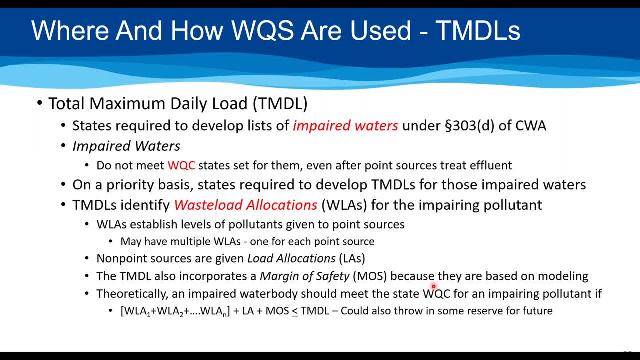 and assessment piece a lot of times feeds right into the tmdls or the total maximum daily loads. and you know the total maximum daily loads come under section 303d of the clean water act and it says that states are required to develop lists of impaired waters. 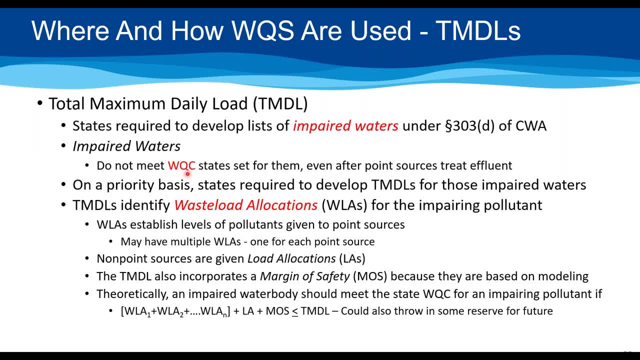 you know impaired waters are, basically they don't beat those water quality criterion that we just talked about. and you know that basically because of that monitoring and assessment work, so it says on a priority base, states you know are required to develop those tmdls to try to. 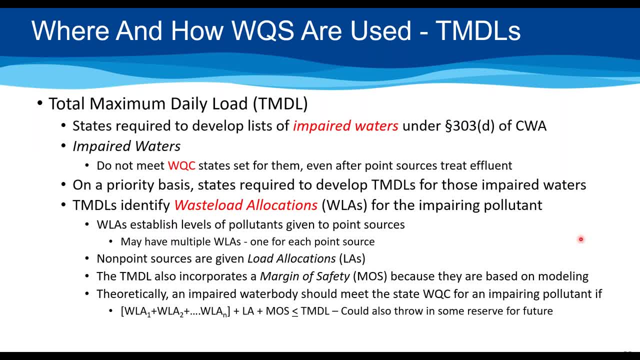 bring a water back into compliance with the water quality criteria, and so tmdls identify waste load allocations called for the appearing pollutant. those are for point sources. think of those as wastewater treatment plants and you might have multiple waste load allocations depending on your water body. 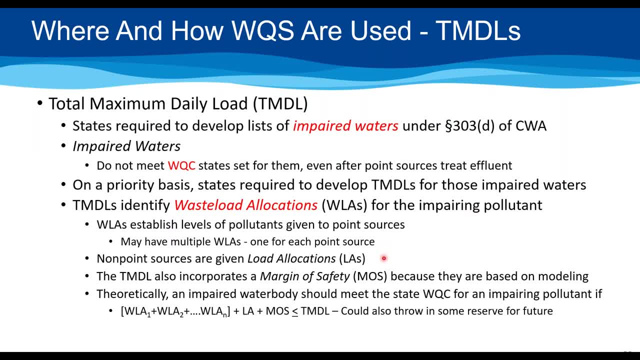 non-fluid. so you're looking at different types of waste load allocations and they're called. and you're looking at different types of waste load allocations that are going to be being used for clean water and you know the tmdl also incorporates, uh, what's called a margin of. 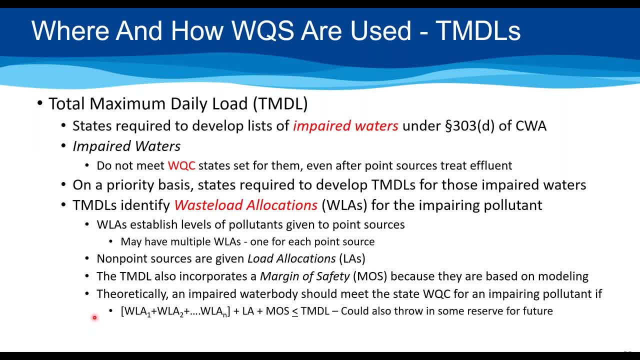 safety, because again, all of this is modeling and non-point pointing and it can be a pretty coarse calculation sometimes. so you throw in a margin of safety and theoretically then if you had all the waste load allocations you could probably throw in a margin of safety. so you're. 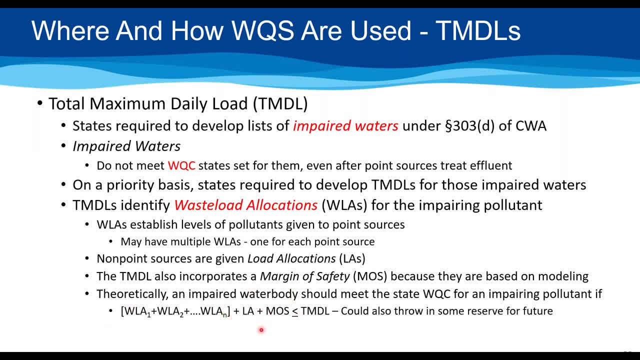 allocations, up all the load allocations and the margin of safety and they turn out to be less than the tmdl, then your water body complies and can probably come off of that impaired waters. and one thing i should add: some states also, particularly in these waste load allocations, will set aside. 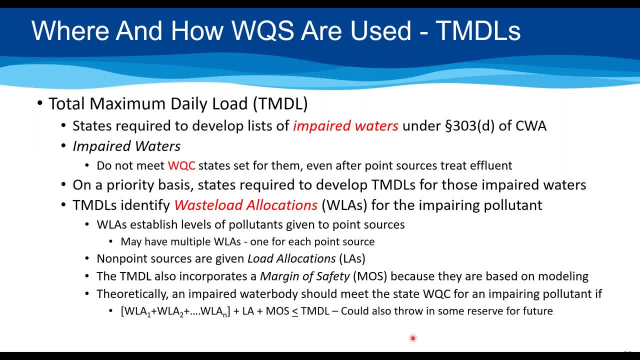 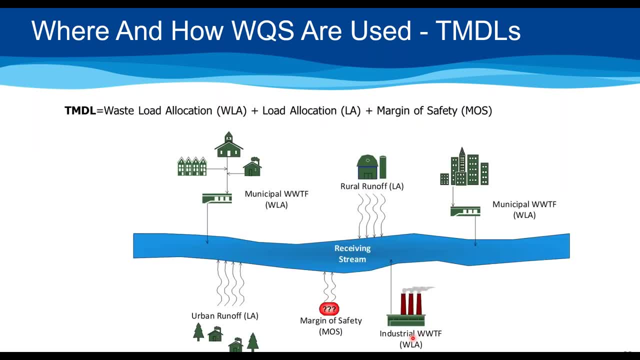 some for a reserve for future growth, in case one of those dischargers needs some additional- uh, waste load again. i like pictures and all this picture tries to show is that you've got these point sources here that discharge into the water body, they're given waste load allocations. you've 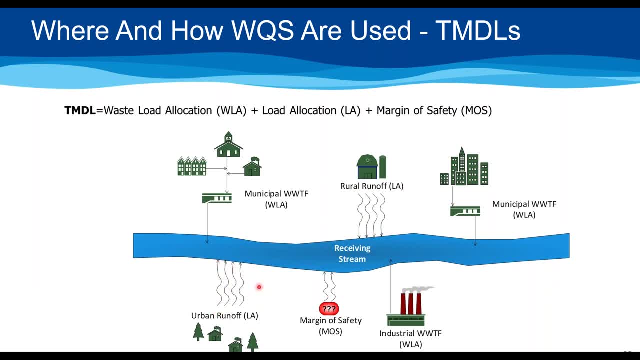 got runoff. you know, as long as it's urban runoff that's not controlled by what's called an ms4 permit, the stormwater permit- it's going to have some kind of an allocation associated with it, and then you get your margin safety and all those things add up to the tmdl. this i thought you know, because i said that you could have multiple. 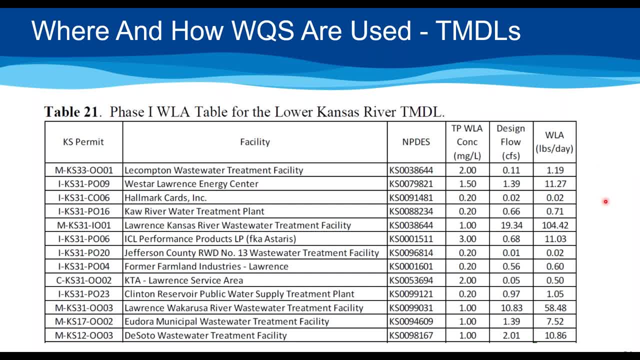 waste load allocations in a water body. this is a table out of the kansas tmdl for total phosphorus for the lower kansas water body, and just to show you that there's all of these dischargers here that have a waste load allocation associated with it. so you've got a lot of players. 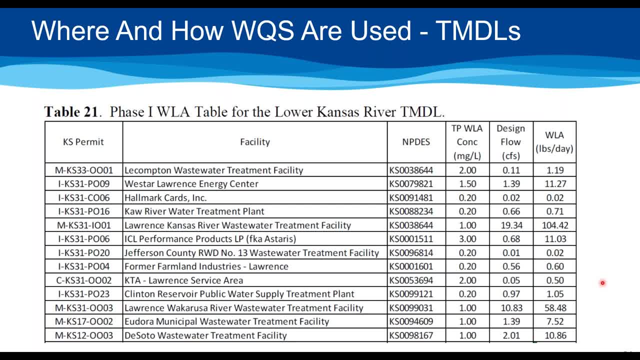 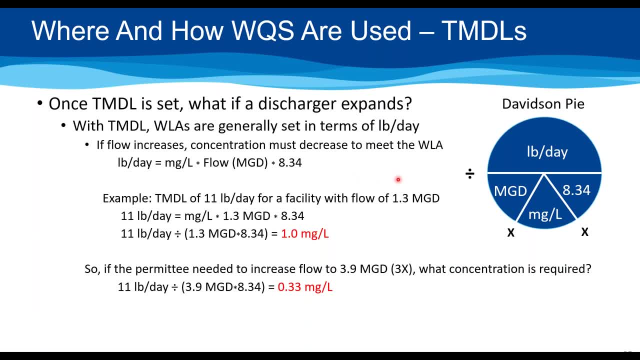 in some of these basins that you're dealing with on the waste load out, and so what happens, you know, once the tmdl set of the discharger expands, okay, well, i know operators are probably familiar with what's called this davidson tie. that, you know, says: well, if i want to do, 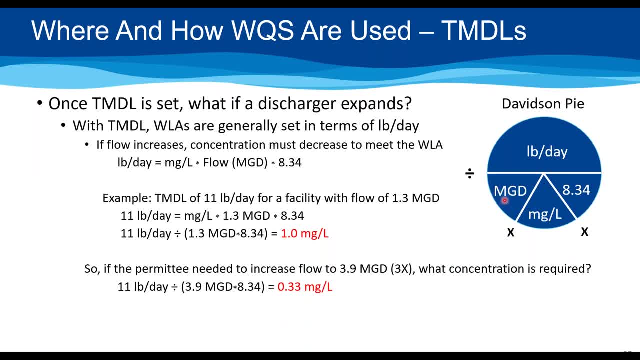 pounds per day. i multiply million gallons per day of flow times milligrams per liter, times 8.34. it's done like that. if you're looking at it the other way, the pounds per day, which is what the tmdl is often written in, it says milligrams per liter to one milligrams per 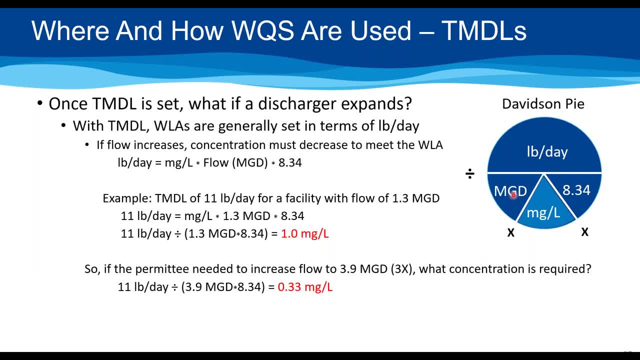 liter. it's pounds per day divided by milligrams per million gallons per day times 8.34. so as an example, let's say that we have a facility that's got 11 pound per day tmdo- okay for a particular pollutant, it's 1.3 million gallons per day. you divide that out, you get okay, that's a million. 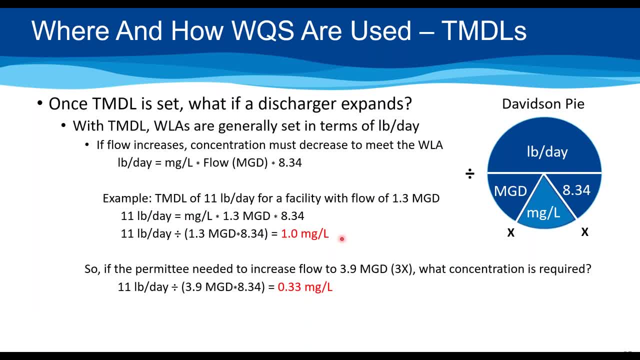 or one milligram per liter, so kind of a permit flip. so if the permittee, though, needed to increase its flow by three times, let's say go up to 3.9, what concentration is required? well, it's going to be the same 11 pounds, because that tmdl has been set. so you get that same 11 pounds. 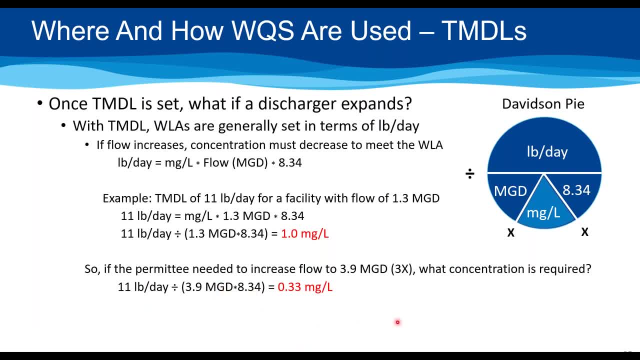 divided by 3.9 times 8.34, which is 0.33. you know a lot of you good with math probably figured out. well, if they up the flow by three times, the concentration has to be divided by three times. so that can get pretty tricky with some pollutants. you can really begin to get the limited technology. 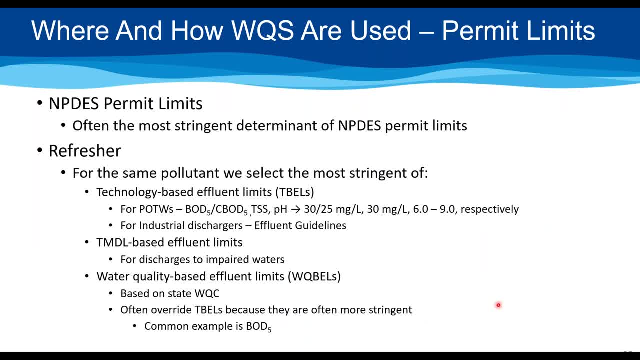 as to what can be done on some of those particular parameters. so, lastly, we're going to talk about how our water quality standards are used. operators, cities, industries typically see, as those are where it is to derive permit limits, and typically the most stringent of the permit limits. 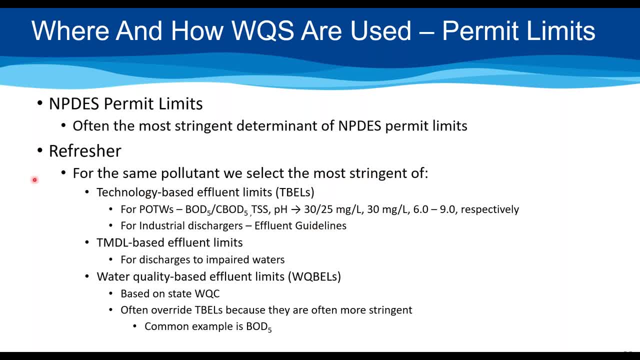 i'm going to give this really short refresher for those who aren't just familiar with the permitting. it's for the same pollutant. we have to select the most stringent of technology-based effluent limits, tmdl-based limits or water quality based limits for potw's or publicly owned treatment works- think of municipal dischargers that you know they. 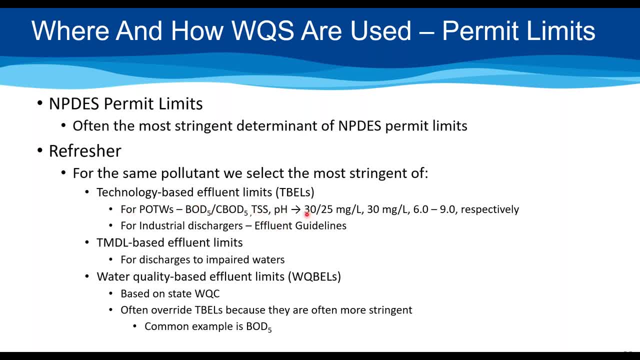 have bod, pss and ph 30 milligrams per liter. bod 30 milligrams per liter solid six to nine ph. industrial users have these guidelines so you'll figure that out. for those dischargers you've kind of got them because they're technology-based. then you've got to look and see if they've got. 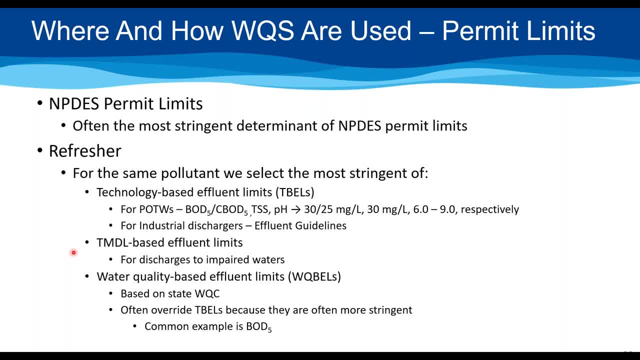 tmdl-based info, but even be all written in the water body where they discharge, and are they given a waste load in the location? if they're in an impaired water, they probably do, so that comes into play. and then, lastly, you have the water quality based effluent limitations. 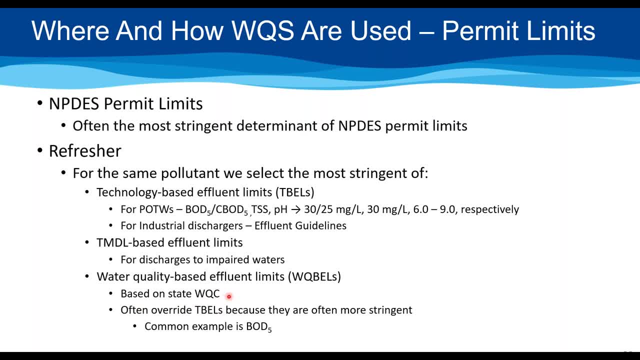 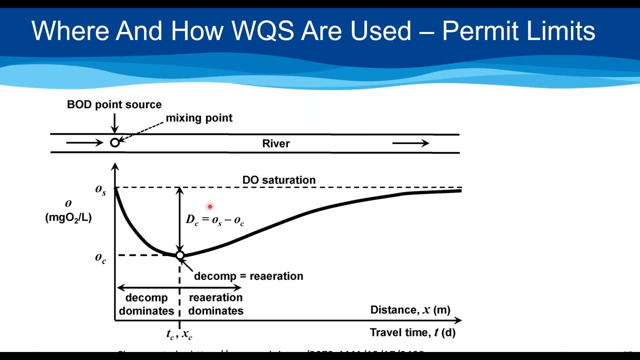 which are based on state water quality criteria, and those very often override those technology-based limits because they tend to be more stringent. and there's the one you see here. that's what's called the flow of oxygen. so it's very well known, but you've got to be a little bit more careful about how to identify. 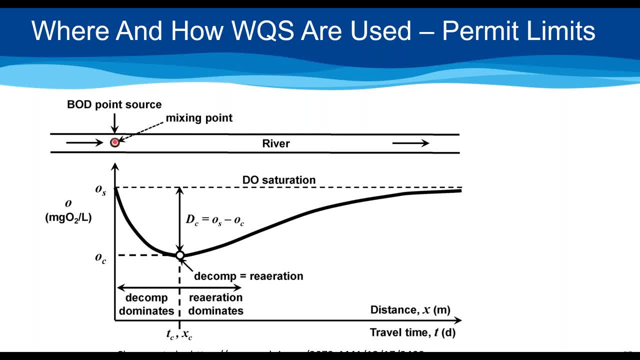 those kinds of things in the water. and then when you're dealing with biologic, you can see it's a little bit more complicated. and then what i'm going to be doing here is i'm going to be taking the rod water. how much will it add up? 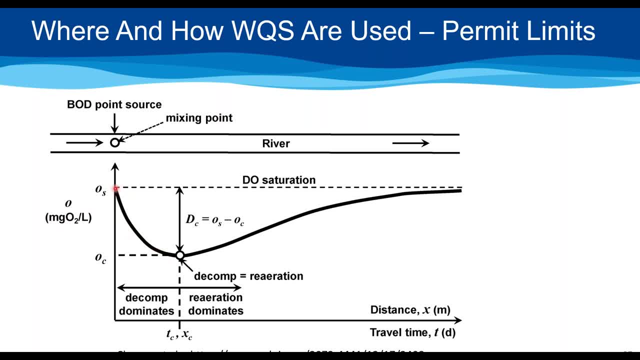 and also i'm going to be taking and then changing the surface of the water on theaction. i've got a little bit more of that as well here: compute dissolved oxygen. so basically it says you drop it in the water and the bugs in the water are going to keep using that food, that organic matter that's in the bod, until it reaches a point. 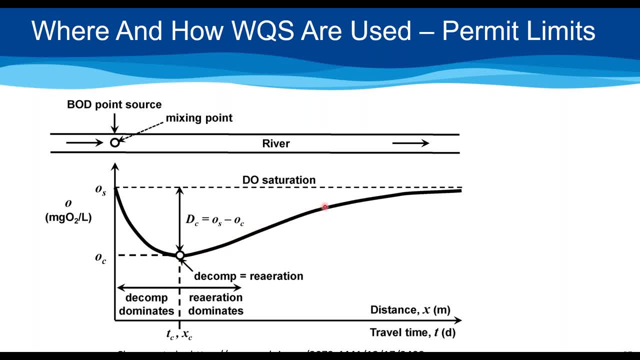 to where the reaeration in the water starts, building the dissolved oxygen back. and so what happens is, if your water quality criterion would happen to be here and you first model it at 30 milligrams per liter of bod, and it bottoms out below that water. 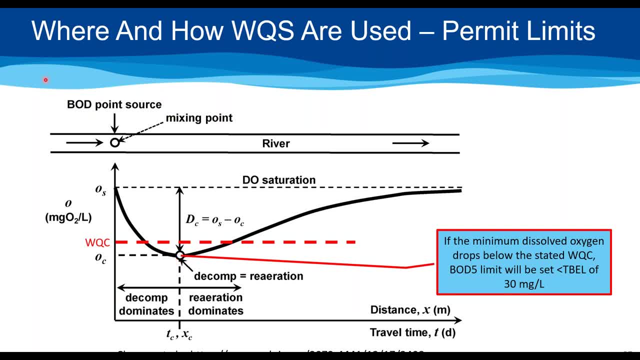 carbon water quality criterion, then you've got to reduce the bod up here at the wastewater plant, and so you'll often see bod limits set anywhere from 5 to 15 milligrams per liter, even though everybody typically sees the technology based limit of 30 milligrams per. and then, if you want, 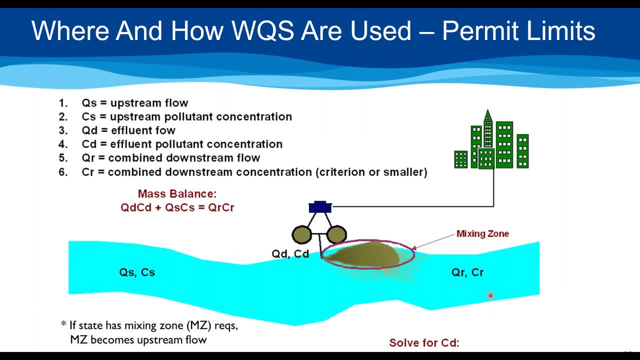 to look at how you can reduce the quantity of the water that's in the water. you're going to have to look at how you can reduce the quantity of the water that's in the water. you're going to have to compute, you know, on a concentration basis for other pollutants. it's a lot simpler than my. 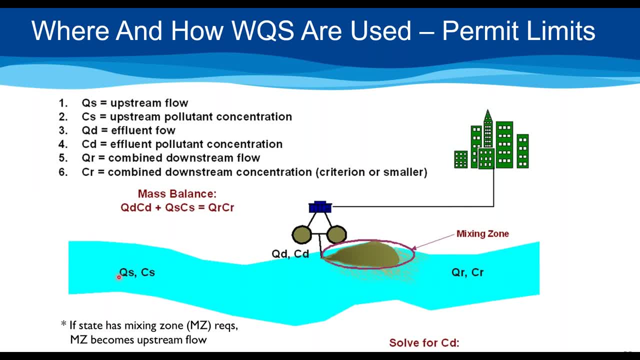 picture looks. i think you know you probably know the upstream flow. hopefully there's a us geological survey gauge. hopefully your monitoring network in your states captured the upstream concentration. you know flow at your wastewater treatment plant. you're trying to figure the concentration that's allowed you've got. 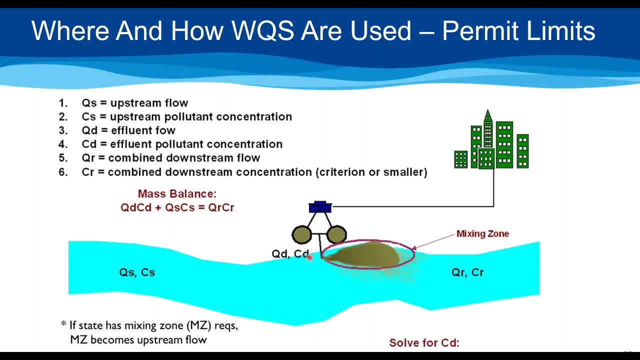 the flow in the river, which is just upstream, plus what's being discharged, and then you have the concentration in the river, which is normally set at the water quality criterion. you just solve that equation. you know what that concentration can be solvent. well, you'll see here. i also, though, have this little area put up here, called the mixing. 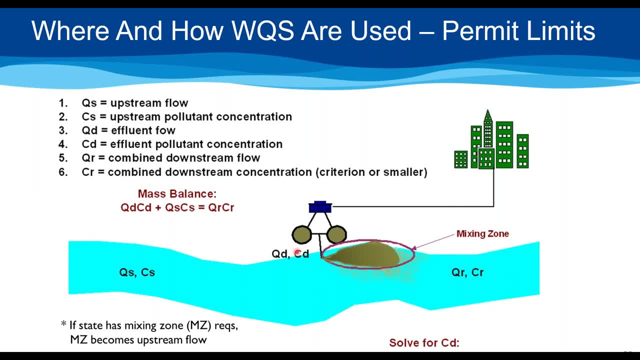 zone. many states will have mixing zones and it will say: you know, you can only mix in 25 percent of the river. maybe it has to be fully mixed within a quarter mile. various things that different states have, and so that can trigger in to how that concentration is made. there's a lot of other things. 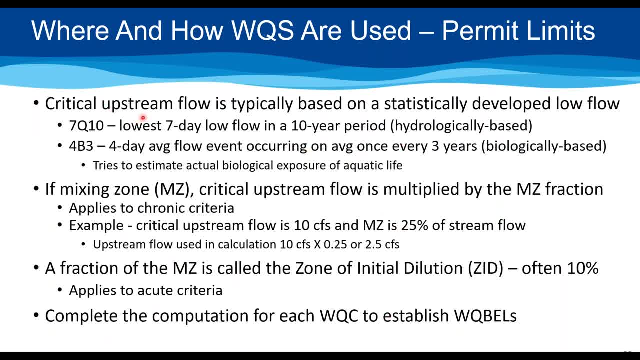 that have to go into, and one of them is: well, what upstream flow do i use? you know i go out, i look at kansas river here near my house, and you know it's up. you know, top of the banks to times i see sandbars. so which one do i use? 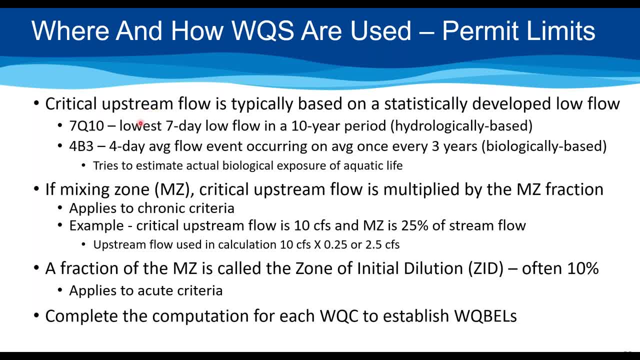 you know it's. you know, top of the banks, to times i see sandbars. so which one do i use? you know it's. you know, top of the banks, to times i see sandbars. so which one do i use? and so it's usually a what's called a critical low flow and the typical low flow, as you see. 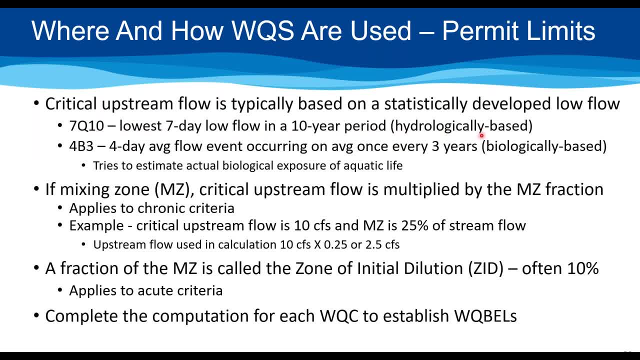 or 7q10, or the lowest seven day flow in a 10-year period and that's hydrologically based. one that's generally preferred is what's called the 4b3, or the four-day biological flow flow, and that's the four-day average that that occurs once every three years and that really tries to 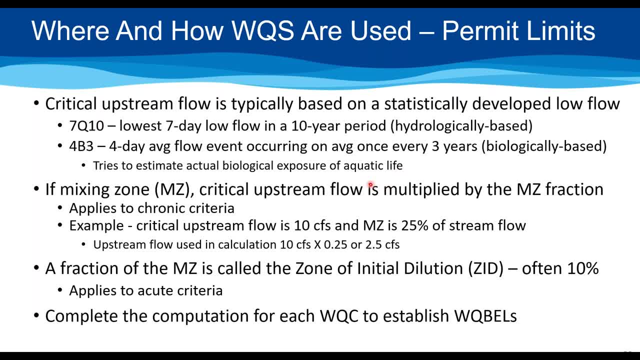 the four-day average that that occurs once every three years and that really tries to estimate the acute biological exposure to aquatic plants. you might have a mixing zone involved, like i've talked about before, that can limit the amount of flow that's used in calculating that limit. mixing zones are used for chronic criteria. 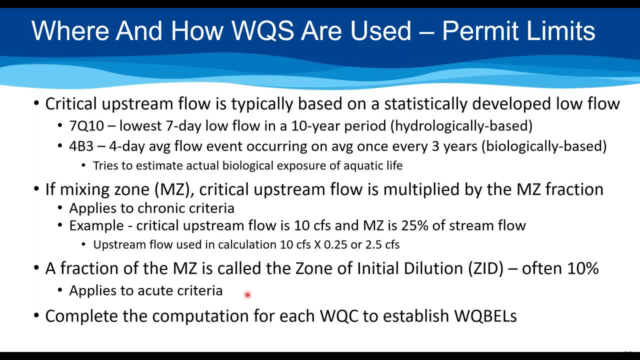 often then you'll use a portion of the mixing zone, which is called the zone of initial dilution. i see a lot of states use 10 percent of that mixing zone and that's where acute criteria block. remember those that are early. so anyway, there's lots of things that go into the computation. 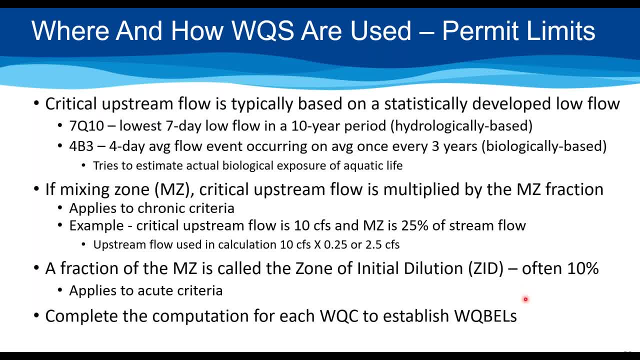 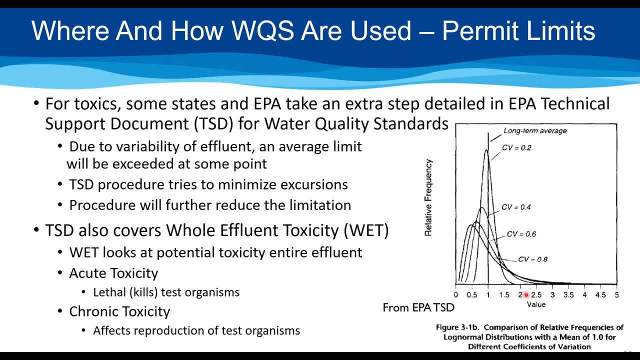 of those water quality based effluent limits, along with just knowing what the water quality criterion is and then to maybe even shave those off some more. remember we've taken the lowest flow and we've done some other things to try to minimize the impact. maybe a mixing zone? 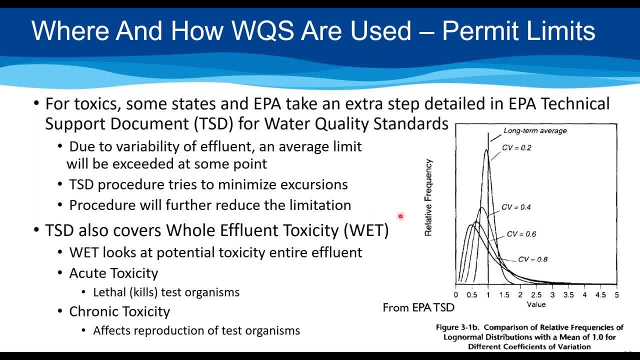 that's what's called the technical support document, which says that you know well, effluent from a discharger can be, you know, pretty variable. if it's not very variable, you get a bell curve type of thing. that looks, you know, most of the data concentrated right here around one. 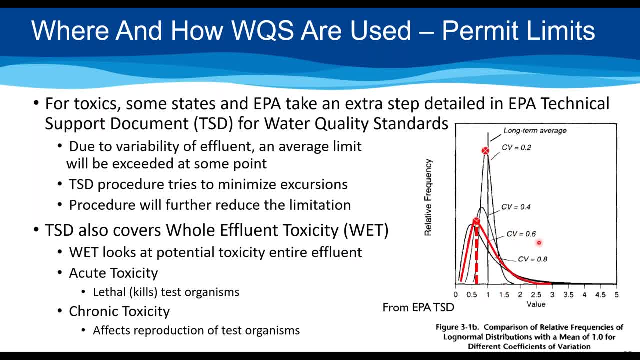 but it says that, well, typically, if you don't know any better- you should use a coefficient of variation of 0.6, and so what that says? at 0.6, that curve looks more something like this: so i'm actually going to move that limit back from one to looks like 0.65.7. 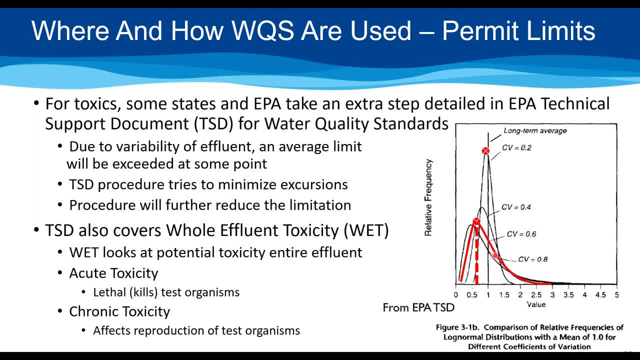 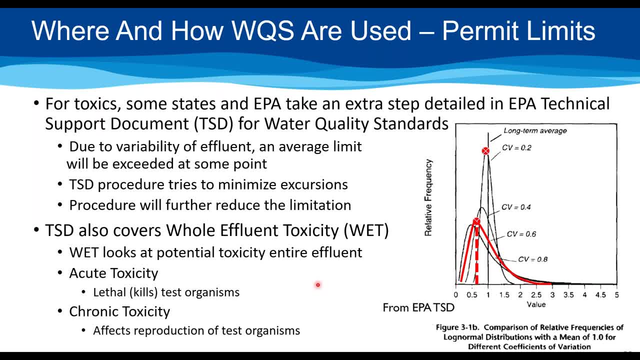 going to be able to do that. so again, some you know things to be fairly conservative in doing that. this technical support document also covers full level of toxicity, which is another criterion you'll find, you know. that's where you actually expose my organisms to effluent and see what happens to them. 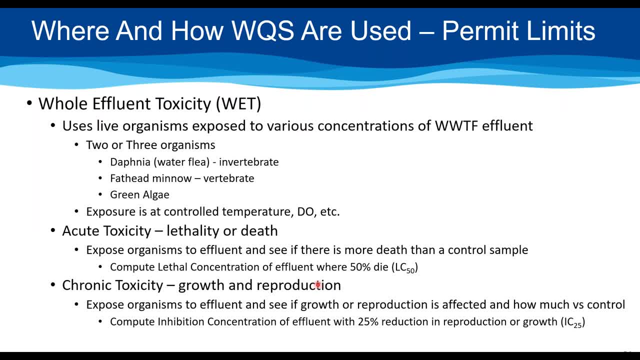 acute toxicity again is kills. the text tests organisms and chronic toxicity is where you have to be careful about that. so it's usually done on two or three organisms. you'll do daphdia quite often to look at invertebrate species- be representative of those- and fathead minnows. 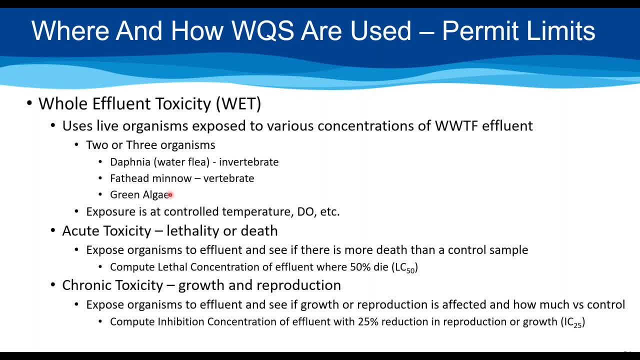 could be vertebrates- recommend you also do something like algae. i don't see too many states that do that and that is, they're controlled in a lab. you take a controlled sample and you expose those organisms and you look and see what they do in terms of survival. 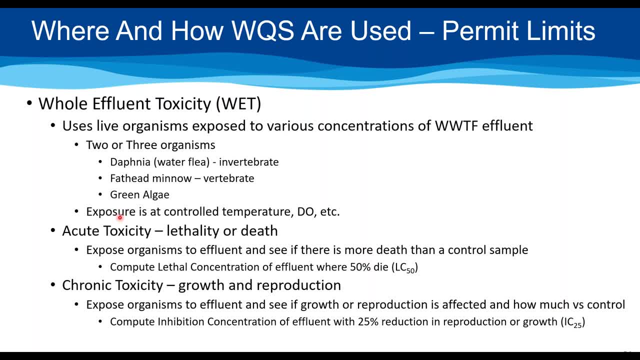 and you can see the changes in their bodies, so the white, and you compare those in the different levels of exposure to network and depending then on what you find, you can have the acute toxicity which is lethality or death and you try to compute what the lethal concentration is for 50 die that can become a permanent limit if the chronic toxicity look at that growth, reproduction, and that you try to compute with this intermission concentration for the 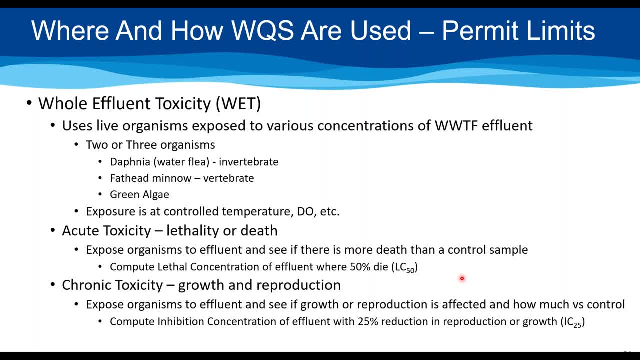 you look at that growth reproduction and that you try to compute with this intermission concentration for the 25% of the organisms is And that can be rolled into the permit limit. Often you'll just see it as a. you know these organisms have to survive or reproduce an x percent of effluent. that's been 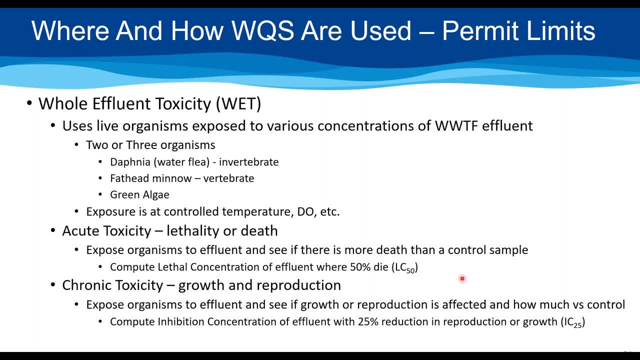 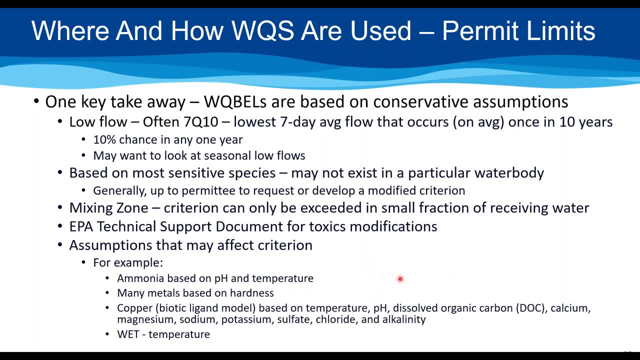 diluted with the remainder, you know, just clean lab water. So you'll find that, And so what I wanted to give you then, on permit limits particularly, is that water quality-based limits are very based on conservative assumptions. That little flow, you know a 10% chance it'll happen. 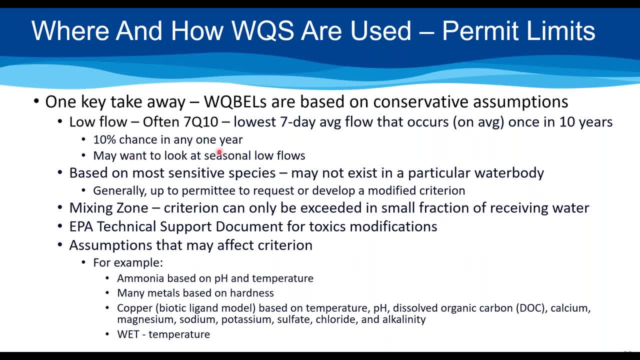 in any one year. You may want to look at seasonal low flows. You can compute low flows as being different winter and summer, or wet and dry season. whatever those happen to be, They're based on the most sensitive species And, as I talked about before, you might want to say those sensitive. 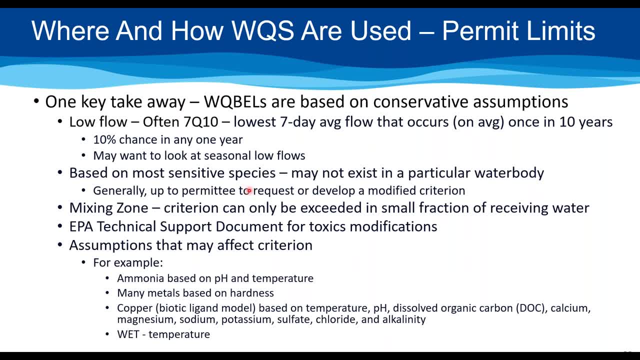 species don't have the most sensitive species You might want to say. those sensitive species don't exist, you know, in my water body. So I'd like them pre-computed and go to criterion. You've got mixing zones thrown in that reduce, you know, the amount of water that's used to, dare say, dilute. 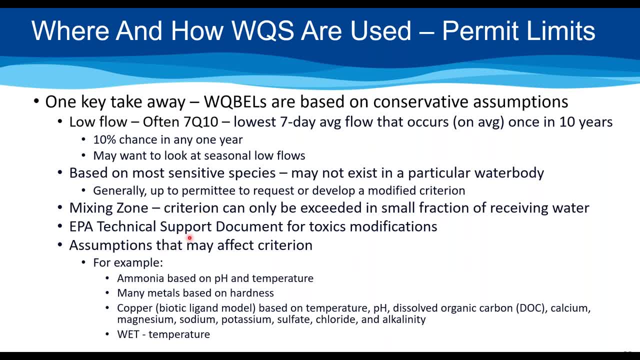 And then you've got that tech support document. you know that can modify and reduce those concentrations for toxics due to the variability of effluent. And then there's a whole lot of assumptions that go into criterion also. Ammonia is based on pH and temperature. Heavy metals are based on hardness. often You've got 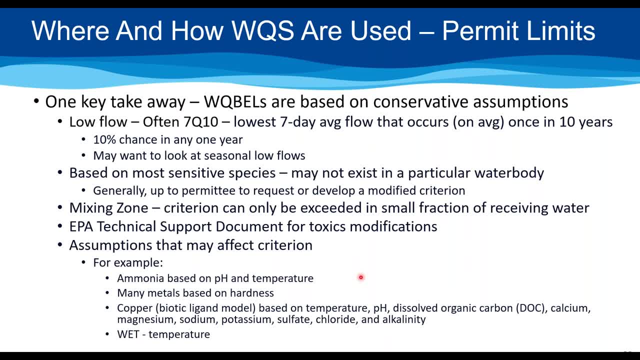 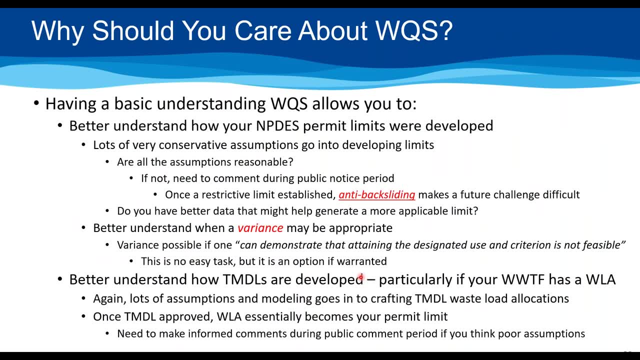 copper, this biotic ligand model that's out there that has this whole string of parameters- you know and you have really good data on that- And the whole effluent toxicity can really be based on temperature. So why do I say this is important to you to know about our quality standards. 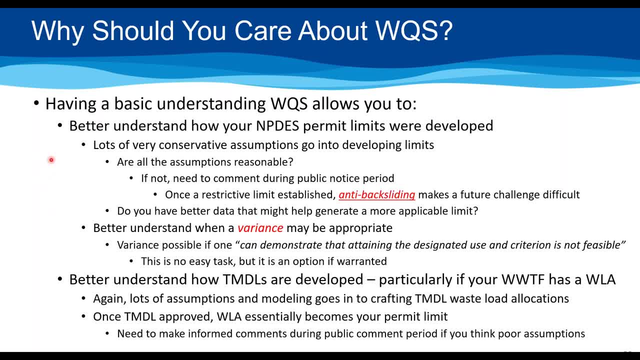 Well, it's just so you can better understand how your NPDES permit limits will develop. Again, I understand there's lots of conservative assumptions and you just want to make sure all those assumptions are reasonable And if they're not, you need a comment during public notice. 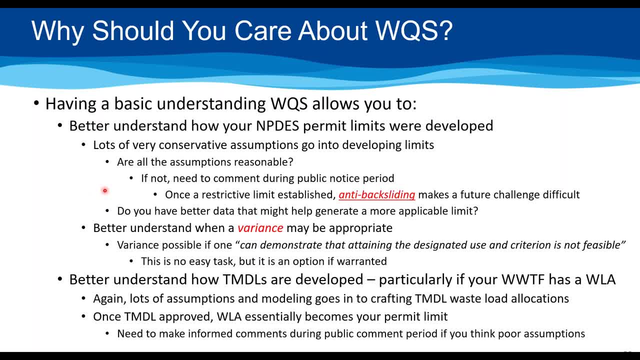 period. You know, hopefully every state's doing a fact sheet, or what's called a statement of basis, that explains the steps they went through and all the assumptions they made for doing that. Ask for that sometime if you're a permittee, and then try to see if you agree with how they came up with those limits. 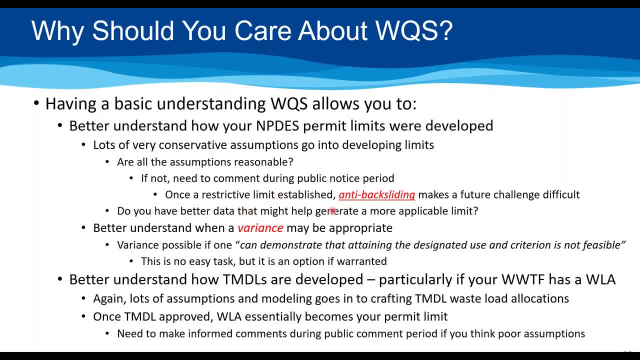 I say that because once a restrictive limit is established, there's a provision of the rules called anti-backsliding which make it a future challenge of a standard difficult. It makes it very hard to increase that value once it's down to oral value Again, it will help you better. 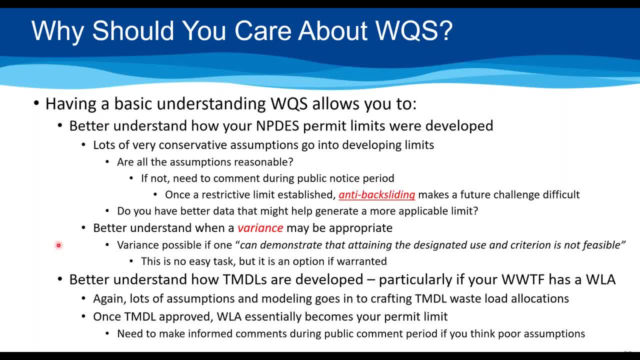 understand what variants might be appropriate If you really just can't meet the criteria, and that is possible. it's not an easy task. As I say, that can be a whole session in itself. Talk about variances and it helps you better understand how TMDLs are developed. 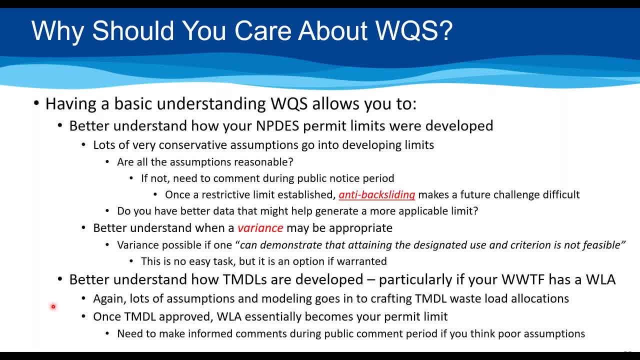 Particularly if you have a waste load allocation associated with the facility, because there are lots of assumptions, lots of things that get into it. I said I'd give you some real world examples. Well, that one I gave you on the TMDL with the facility. it's the best way to get. 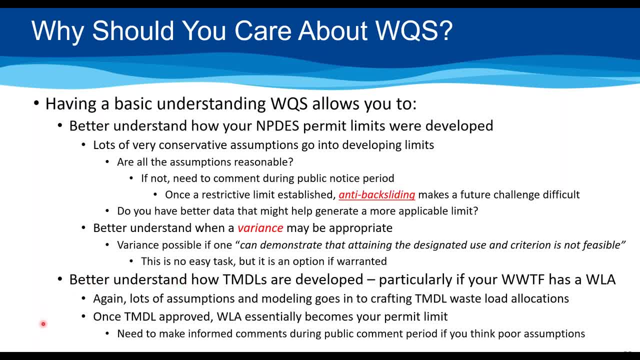 it into the facility. It's not a very practical data. It's not a very practical data. And if you're looking at the one here in Kansas that recently had a industry being built that is a $4 billion with a B plant, low flow- now they get this big industry that uh has a lot more flow that they have to treat. but 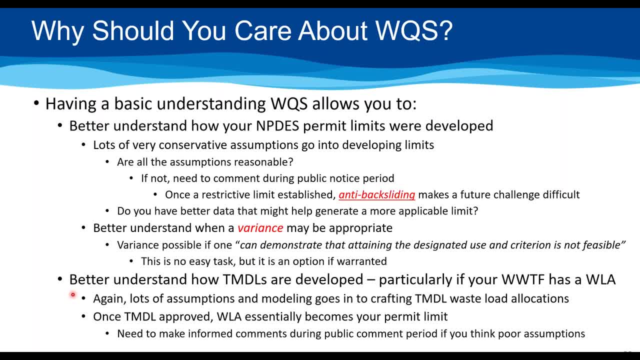 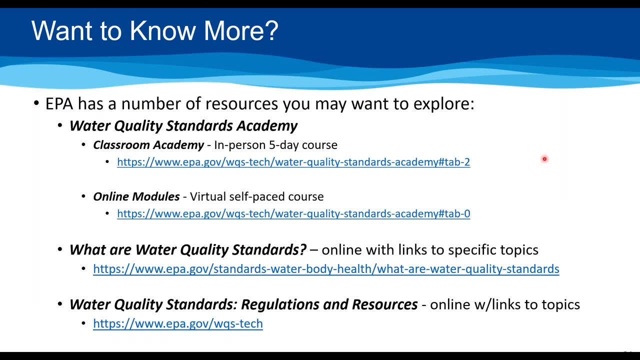 they're locked in on that tmdl mass so they have to meet a very stringent permit limit. you know, had they known this was going on up front when the tmbl was established, they maybe put a comment on that. so, um, hopefully i've given you a very compressed uh, very quick uh- review of what 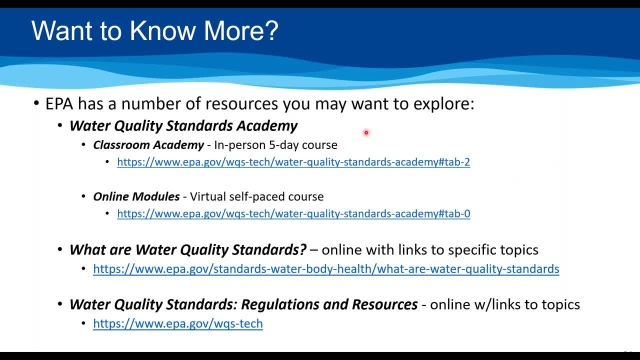 standards are. if you want to know more, there's a lot of resources out there. you've got epa's water quality standards academy. again, it's in person in a five-day course. they don't think they're offering that very often these days, but it is out there. they have taken a lot of those. 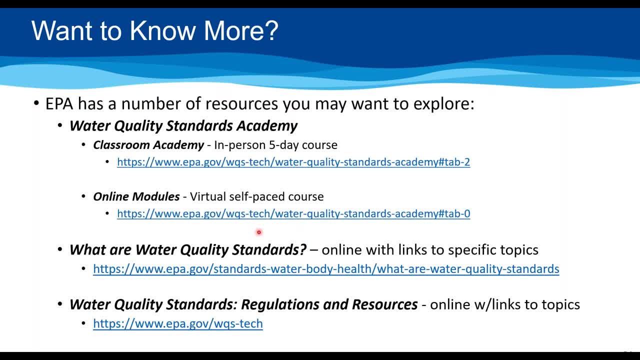 and turned them into online modules so you can take your own self-paced water quality standards academy if you would. there's a link to that. epa's main webpage has a good explanation of what our quality standards are and then links into specific topics, and then they've also got a regulations and resource with online links- topics at that link and 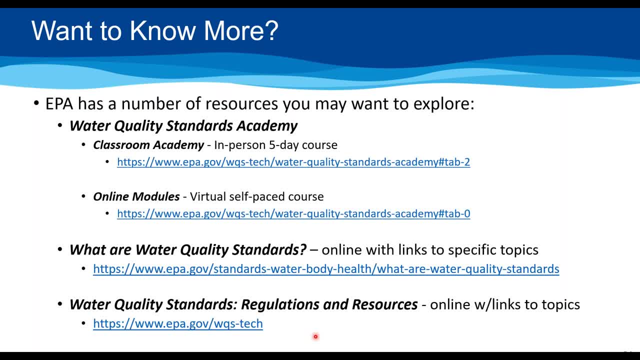 it's one of the things that you know. i think if i fascinating, it's like i mentioned, anti-degradation probably doesn't even take up one page in the regulation book. i think the last time i looked there were close to 800 pages of guidance, explanatory information out there. 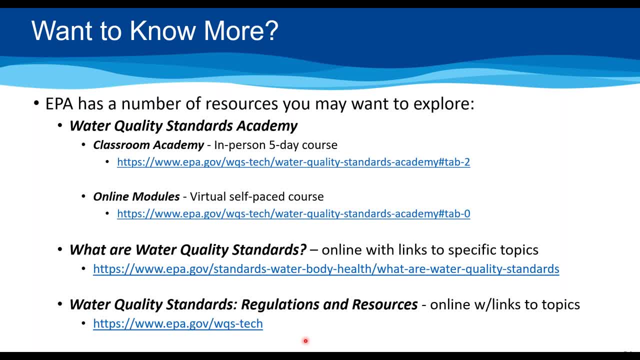 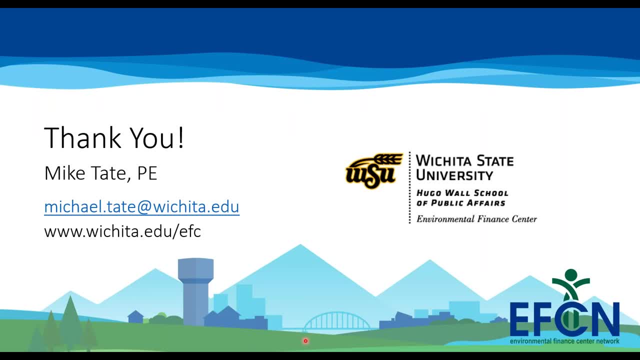 why it may not look like much of a rule in books. there's been a lot of history behind it, so with that, uh, i could intentionally run out the time, but i'm uh welcome, kristen. if we can, i will stay as long as anybody wants and try to answer questions. 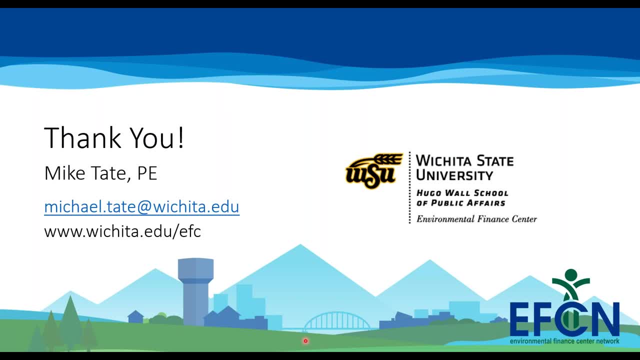 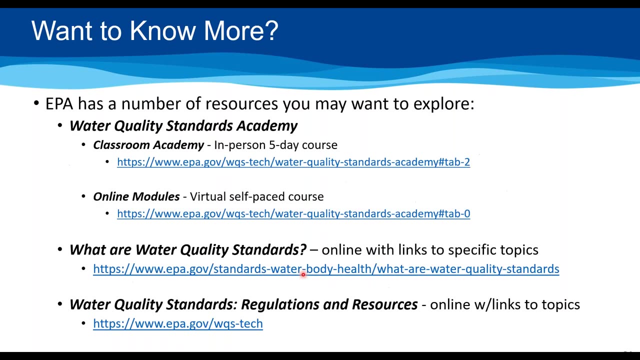 um, karen's got a question in the chat, yeah, so go ahead and get those questions in if you have any. we have only received one so far, mike. it was at the beginning of the webinar. someone asks: how can a narrative criteria be turned into a numeric criteria? 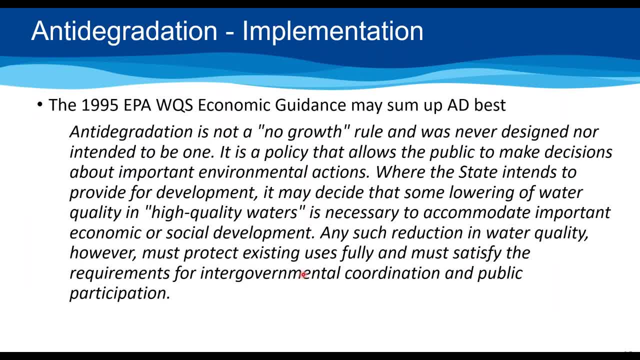 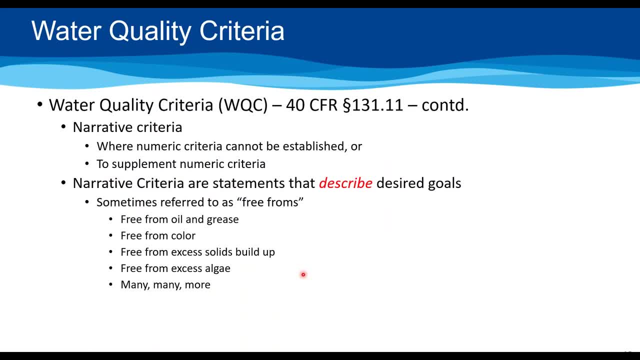 it's a really great question. uh, it's. uh, You know you could do tests on your own. say, oil and grease. people have put different levels of oil and grease in water and see where they believe there's a sheen. Quite often it was used for that. 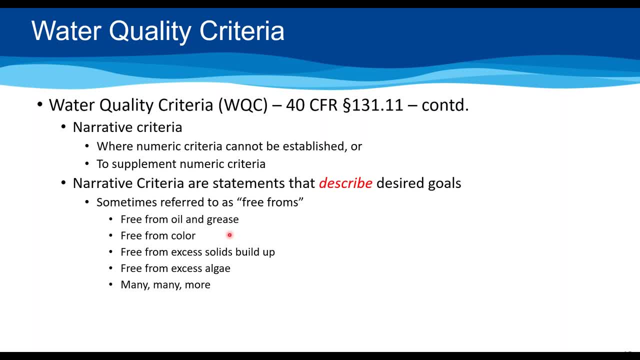 You know color. there are actually color scales out there you can use for water. I find it kind of interesting because there's a lot these days on ways you can come up with narratives for nutrients and then convert your narrative to a number and you know. 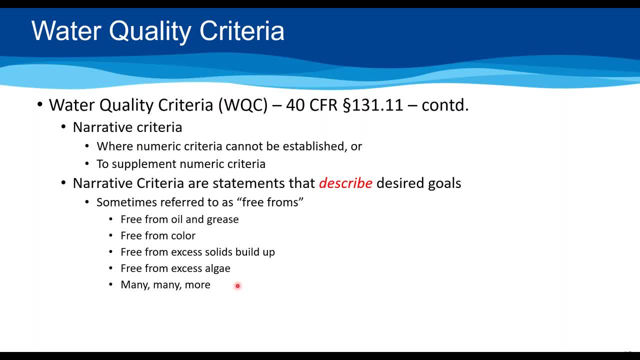 if you can do that, then you've probably done most all the work that's involved in either aquatic life analysis or some type of recreational analysis that would establish the number anyway. So yeah, I think it's always kind of hard when people tell you: oh, just convert your. 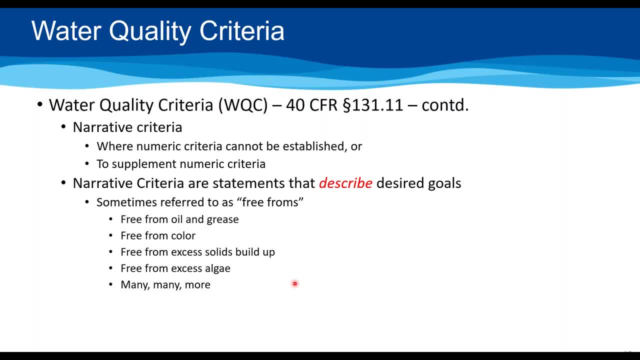 narrative to a numeric. To me, you're basically just doing the work that would be done to create a numeric. Awesome, Thank you, Mike. That's a great question, by the way, because it happens quite often. We haven't received any other questions.